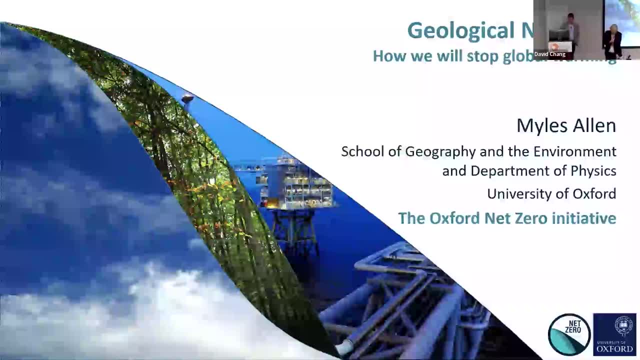 And he's the director of Oxford Net Zero Initiative. He's described by the BBC as the physicist behind net zero And he's been saying He's been studying how human activities and natural drivers contribute to changes in global climate and weather ever since the 1990s. 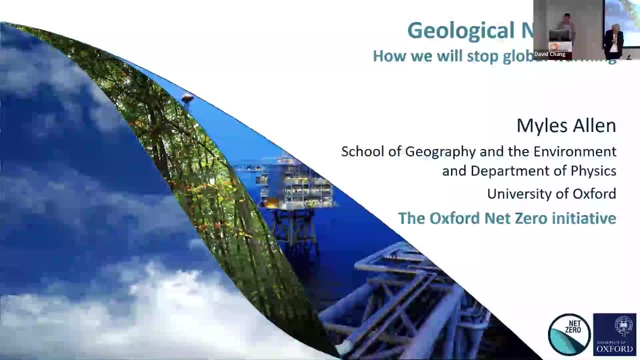 And in 2005,, Miles first proposed the concept of global carbon budget, that peak warming is largely determined by the total amount of carbon dioxide we release into the atmosphere, not the rate of emissions or the atmospheric concentration in any given year. He's long argued that fossil fuel producers should be central to the solution to climate change, rather than just part of the problem. 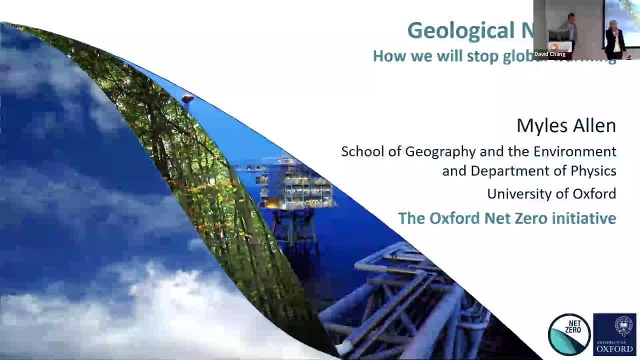 Which calls for policy innovation, and Miles has a TED talk on this that I highly recommend. It's a brilliant TED talk. So he's been awarded the Appleton Medal and Prize for the Institute of Physics and, in 2022, a commander of the British government. 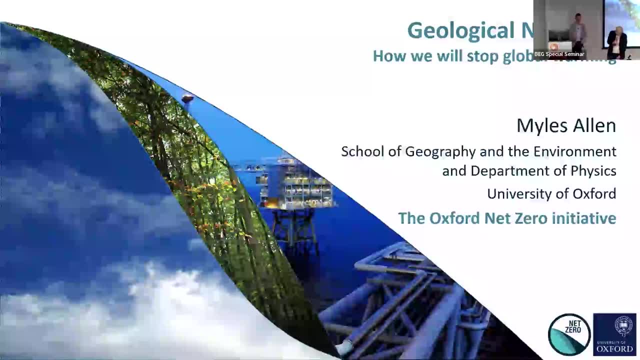 Don't mention that in Texas, Yeah, for services to climate change prediction. So thank you so much. Let's give him a warm welcome. Thank you, Miles. Thank you, Yes. no, we do go into a slightly ridiculous titles in the UK, Anyway, but it's great to be here. 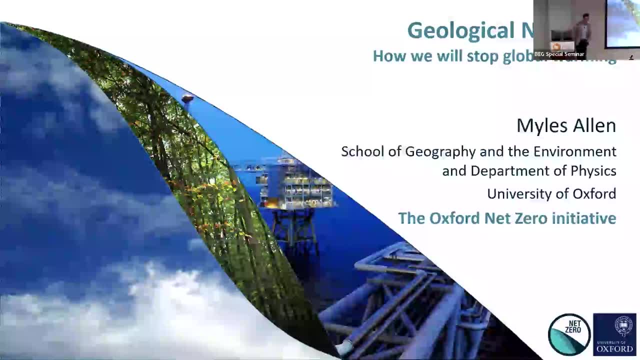 And great, Great. Thank you very much, Catherine, for the invitation And thank you very much everybody who came and talked to me this morning, because I've had a really fascinating morning and it's been great to see the breadth and diversity of work that's going on here. 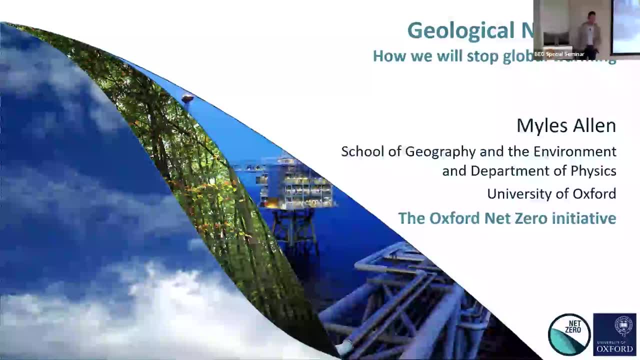 But I'm particularly excited to give this talk in Texas, because I'm convinced that Texas is perhaps one of the- you know, probably one of the- peakiest countries in the world, as a matter of fact. Well, actually, it's either Texas or Norway, would be my guess as to what's going to, which is going to be the first jurisdiction in the world to achieve geological net zero, which is how, ultimately, the world will stop global warming. 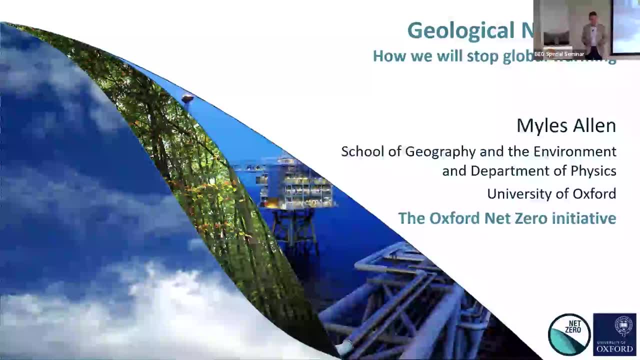 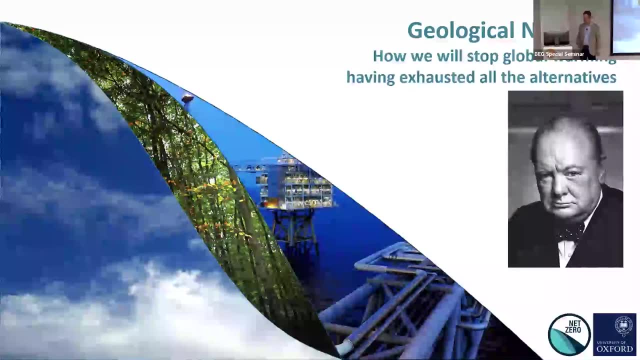 Again to- My punch line has already been spoiled slightly from from you seeing the slides, But, to misquote, exhausted all the alternatives, And so I feel about this particular approach to dealing with climate change. It is how we will ultimately stop global warming after we've exhausted all. 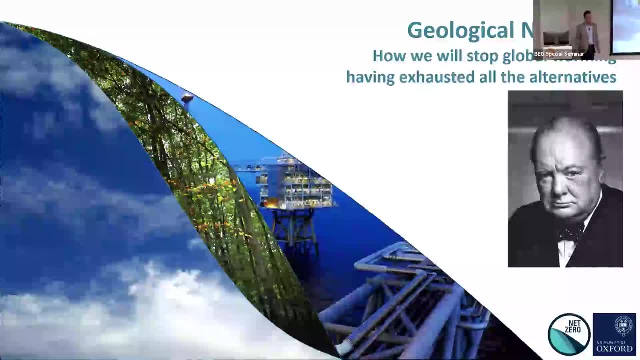 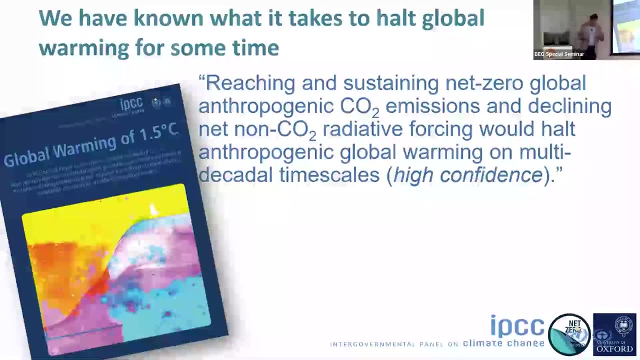 the alternatives At the moment. the sort of approach to dealing with climate change that I'm going to be talking to you about is very, very different from most ways in which governments and academics and everybody else, certainly civil society- frames the problem. Let's get back to 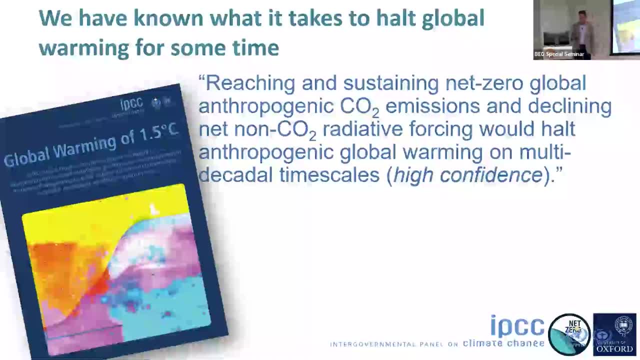 just some basics And we know what it takes to halt global warming. This is the statement in the IPCC's 1.5 degrees report, which I was heavily involved in, And whenever you see these rather sort of tortured sentences in IPCC reports, you know that some people spent a whole night. 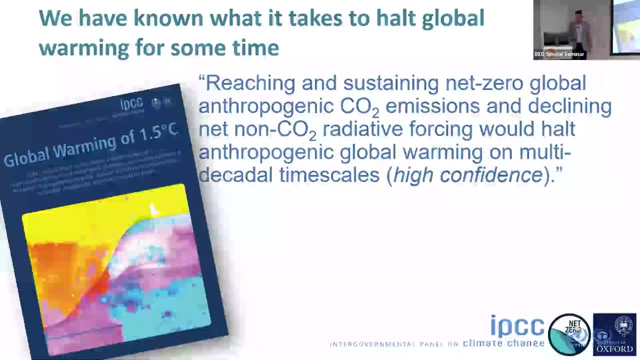 negotiating the wording And that's why it was originally stopped global warming. but that was too much for some countries, So we ended up with halt global warming and things like that. But the sort of jargon in here: human-induced CO2 emissions- you know what we mean by that- And net non-CO2. 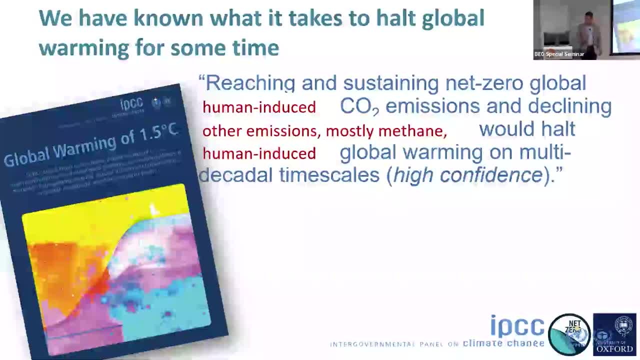 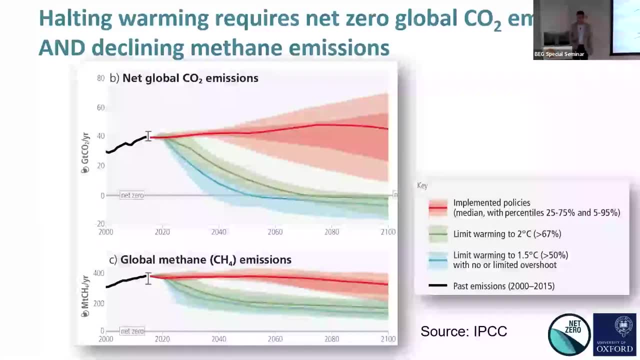 radiative forcing just basically means other emissions, mostly methane. I'm going to be focused on CO2,, though, because we require net zero CO2 emissions and declining methane emissions to achieve the Paris Agreement goals of stopping global warming, That reduction in methane emissions. 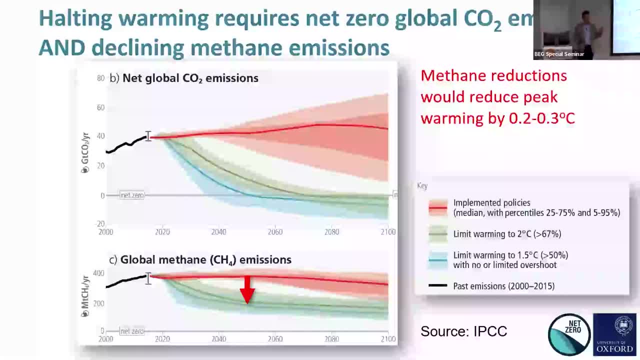 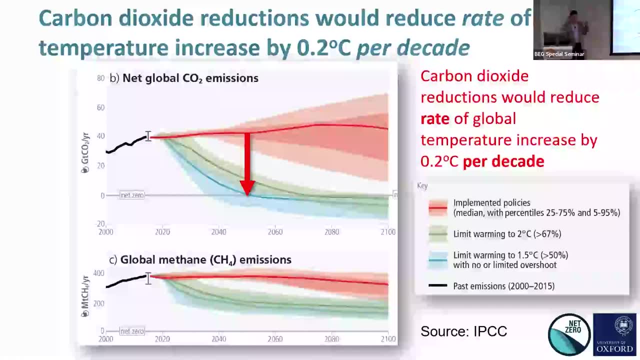 would reduce peak warming by a couple of percent, And that's why I'm talking about the global warming rate, which is a couple of tenths of a degree, which, of course, is important, it's valuable, But just to put this in context, that reduction in carbon dioxide emissions would reduce. 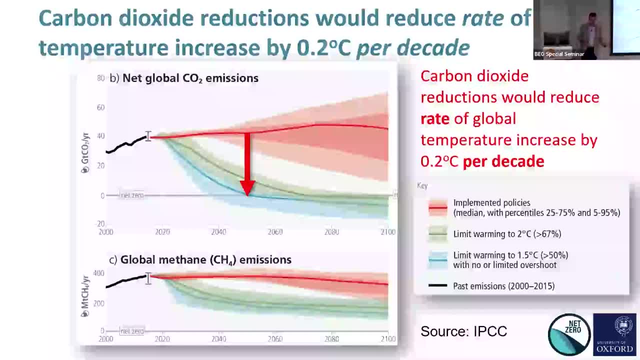 the rate of global warming by two tenths of a degree per decade. So it's really important, particularly as the oil and gas industry is talking a lot about methane at the moment and how they're going to address their methane emissions- And I was hearing that apparently. 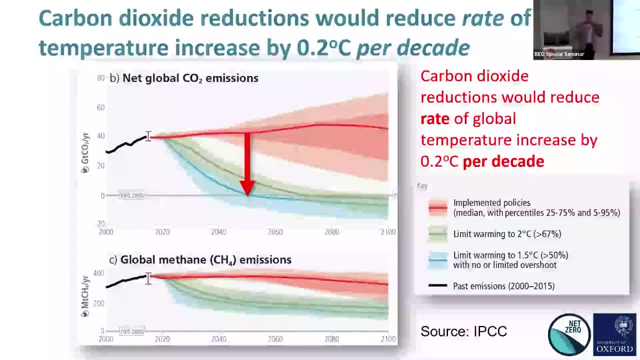 in the Permian Basin there's still some methane intensities of 10% or so, which is pretty desperate. Clearly that's got to be cleaned up, But at the end of the day, this is a carbon dioxide problem. This talk is going to be about carbon dioxide. Where are we? at One and a quarter degrees? 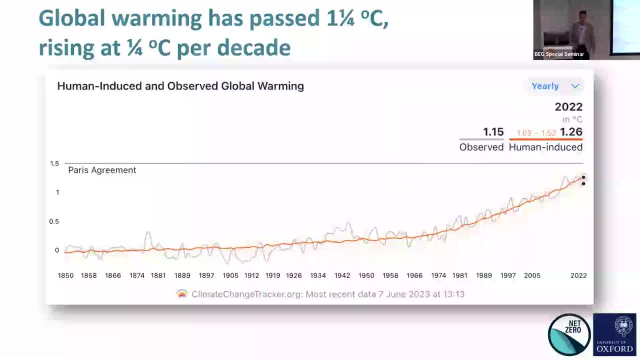 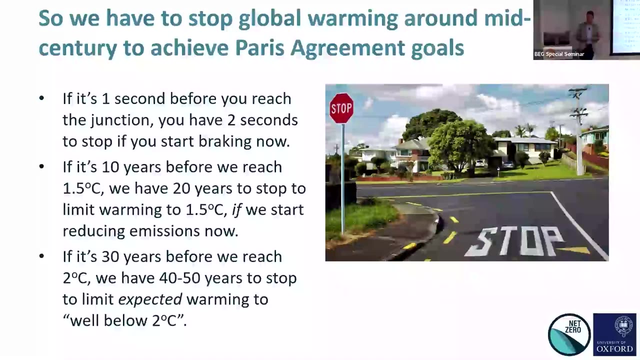 Celsius- I'm sorry, I use Celsius all the time- And we're warming at a quarter of a degree per decade. So it's nice round numbers And we know, therefore, what it takes to meet Paris Agreement goals. Again, it's simply your driving test. You know if it's one second before you get to the 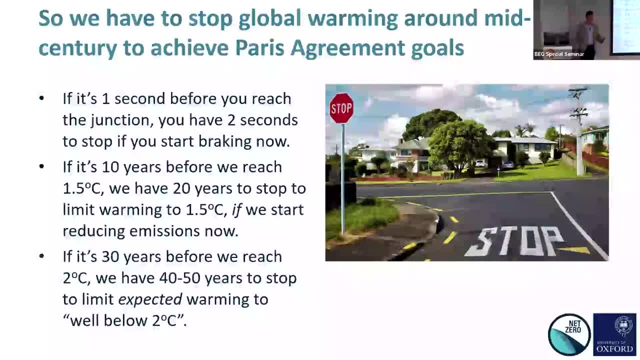 junction, you've got two seconds to stop, only if you start braking immediately. If it's 10 years before you get to 1.5 degrees, you've got 20 years to stop the warming. So that's why we know to meet. 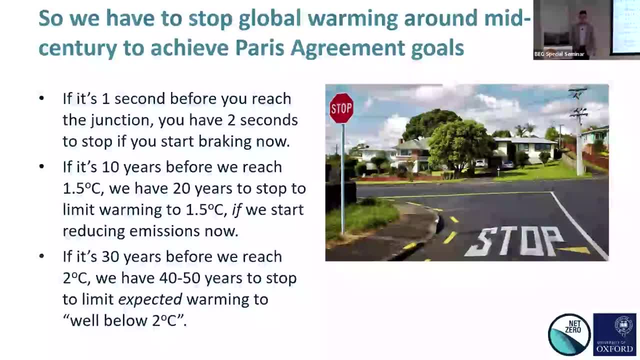 the Paris Agreement goals of well below 2 degrees, pursuing efforts to 1.5 degrees. we've got to stop global warming sometime around mid-century. I think it's really important that one of the conversations I was having this morning was about how many people feel it's too late And there's a 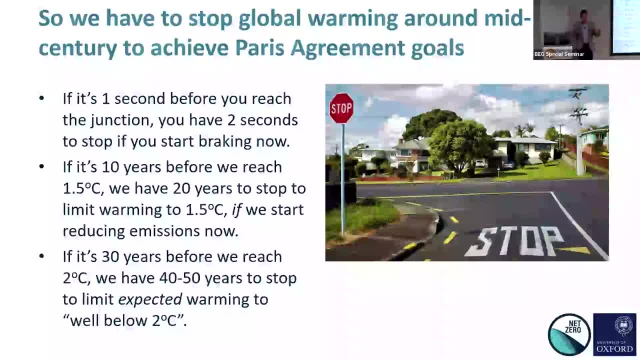 lot of talk, that 1.5 in particular is focused on the fact that, well, we've missed 1.5, so we should give up. I mean no, We need to stop global warming as soon as possible. If we manage to stop global. 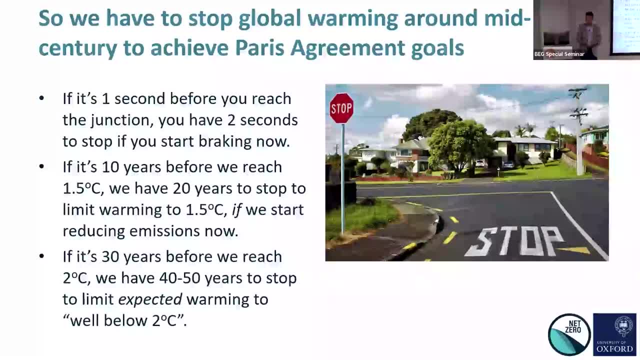 warming around mid-century, we will limit it to pretty close to 1.5.. That would be a huge result. compared to the alternative. It might not be enough to limit it to exactly 1.5.. But at the end of the day temperatures fluctuate by tenths of a degree anyway from decade to decade. So I think getting 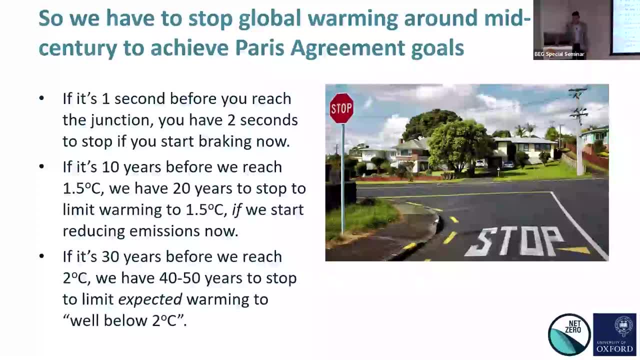 too hung up on. that is a mistake at this point. And again, just to remind you, of course the Paris Agreement did not actually say we were going to limit warming to 1.5. It was pursue efforts to limit warming to 1.5. And the real commitment is to keep it well below 2. And that we definitely. 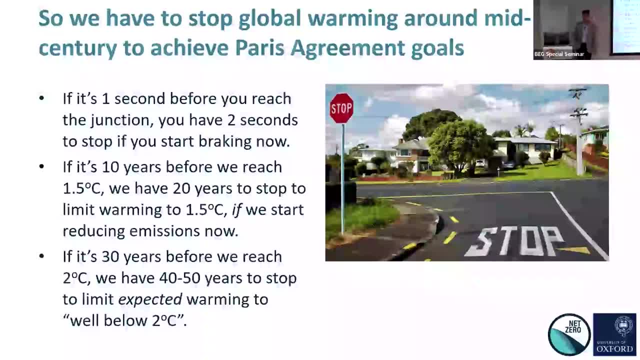 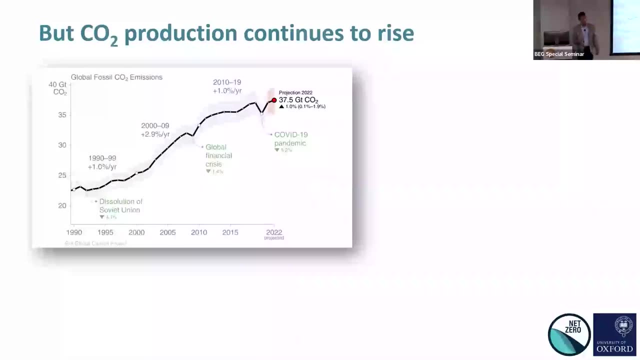 can do. If we can stop the warming before 2070, it'll be. And if we start reducing emissions now, stop the warming well below. But the problem of course we know what we need to do, We're not doing it. CO2 production. 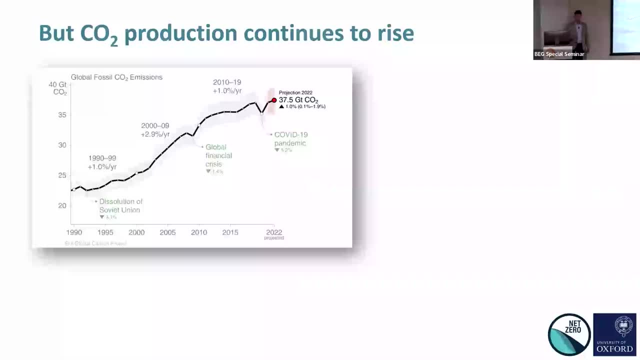 continues to rise. That's global fossil fuel emissions. And notice that this doesn't go to zero. If I showed you what a 1.5 degree trajectory looks like, it's that. So notice the COVID notch there. Basically, to limit warming to 1.5 degrees, we just need to keep going in a straight line. 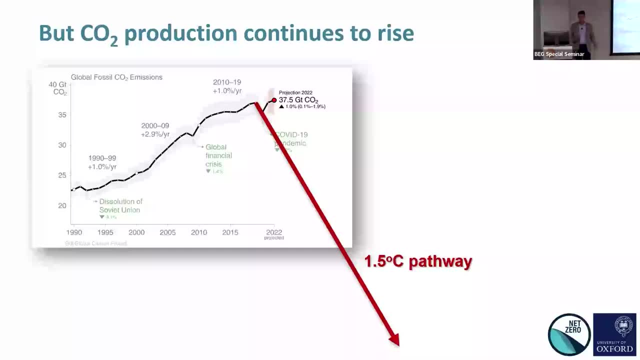 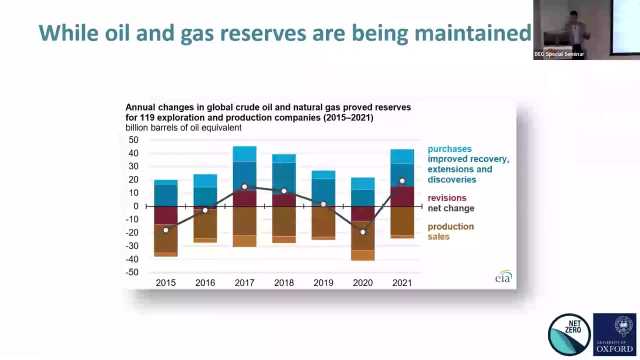 following down the COVID reduction, So you can imagine how disruptive that would be for the global economy. And we are seeing. in the meantime, oil and gas reserves are being maintained, The oil and gas industry is keeping up its reserves And this remains a highly contentious 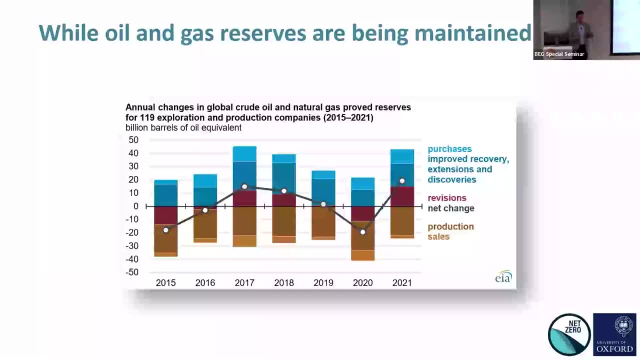 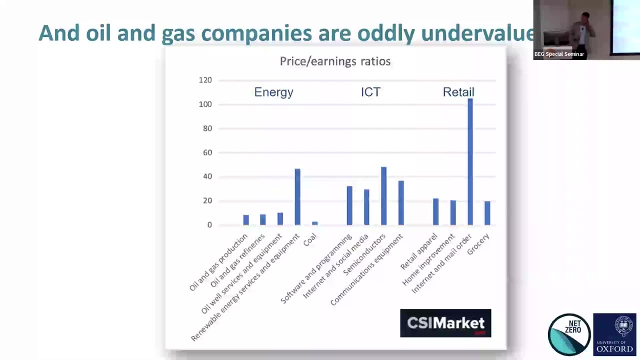 topic. I'll be coming back to this. So in the UK it's becoming highly political whether licensing of new oil and gas extraction In a very unhelpful way. A really interesting statistic that I came across recently was the valuation of companies in different sectors. And despite the fact- perhaps because of the fact- 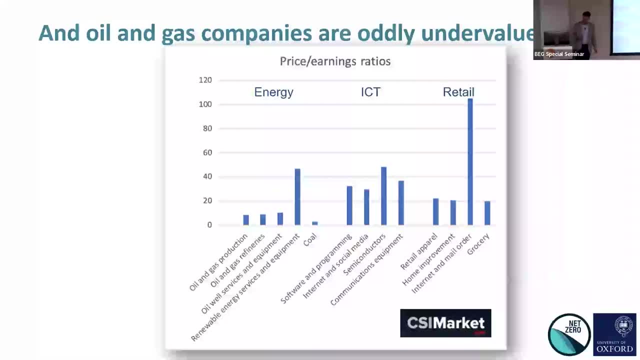 they're making such huge profits. oil and gas production is, in terms of price earnings ratios of these companies, strangely undervalued. The valuation investors place on oil and gas companies is much less than would make sense given the amount of money they're making. You know you compare an oil and gas production or refining. 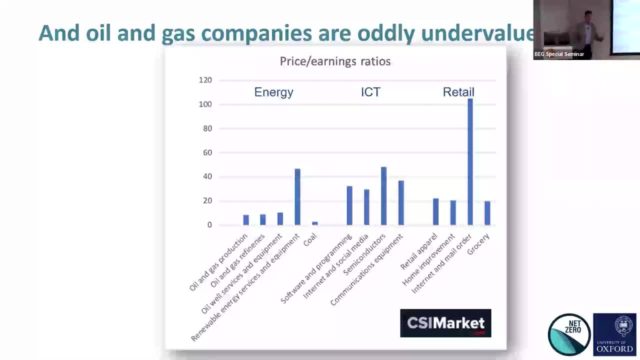 company with. you know a home improvement company, you know B&Q or what is it? Home Depot. So the home improvement company is much more valuable relative to its profits, which is- which is it's interesting- It's the market valuing the oil and gas industry in this way. 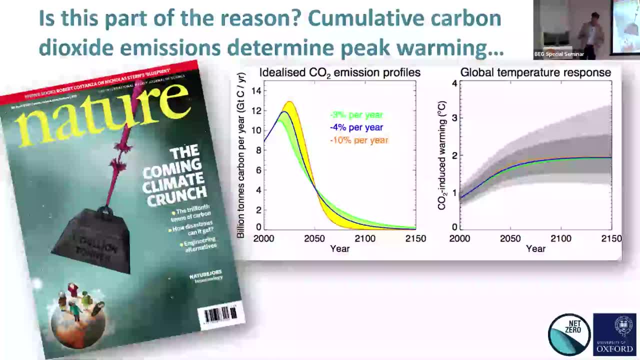 And you know, a question to ask ourselves is whether this is part of the reason, as it were. am I part of the reason? I'm not sure that I would flatter myself with that, But I mean, back in 2009,, we arrived at this conclusion that, in order to stop warming, that it was the total amount of carbon dioxide we dump in the atmosphere that determines. 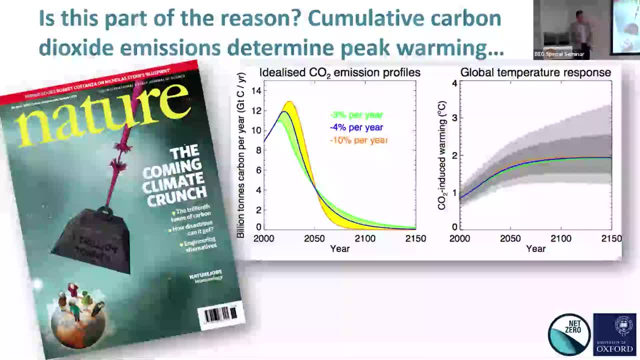 what temperature we get to And that, therefore, in order to stop global warming, we need to reduce global carbon dioxide emissions to net zero. And you'll notice in this schematic here we've got three emission profiles. They all have the same integral under the curve. 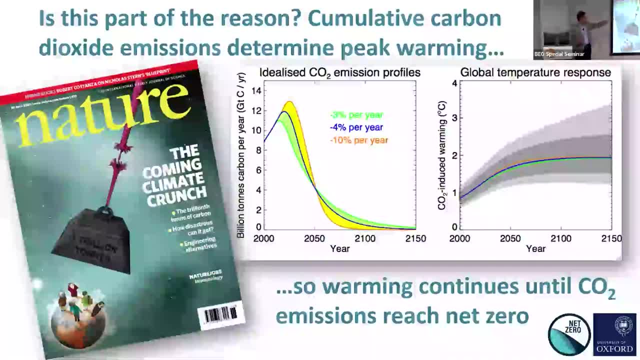 So the same total amount of carbon dioxide is dumped in the atmosphere. They all end up at the same temperature And the differences between them are tiny compared to the uncertainty and the response. So it's not the rate at which we put carbon dioxide. 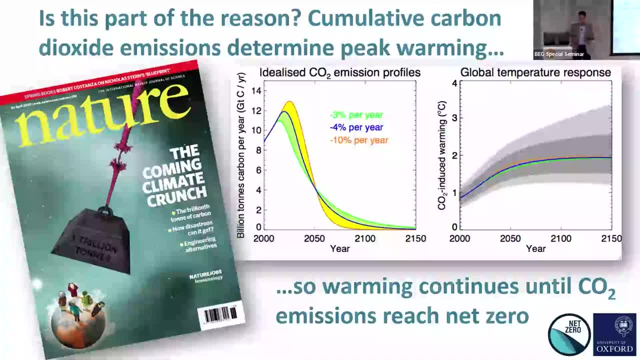 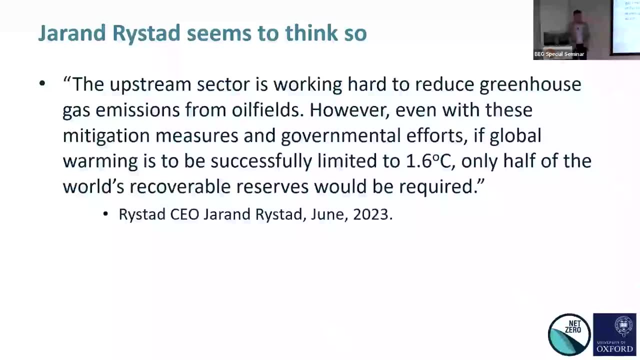 It's the total amount, Which means, of course, that the likes of Jaron Reistad of Reistad Energy- so certainly no environmental NGO- is saying: even with these mitigation measures, if global warming is to be successfully limited to 1.6 degrees- I'm not quite sure why he said 1.6 here- only half of the world's recoverable reserves would be required. 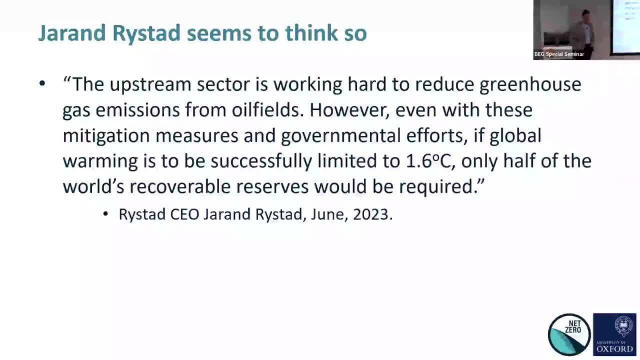 And the question is: are investors? Are investors in the oil and gas industry looking at statements like that and saying: is there something wrong with this industry that at some point we're suddenly going to end up with a whole lot of stranded oil and gas fields? 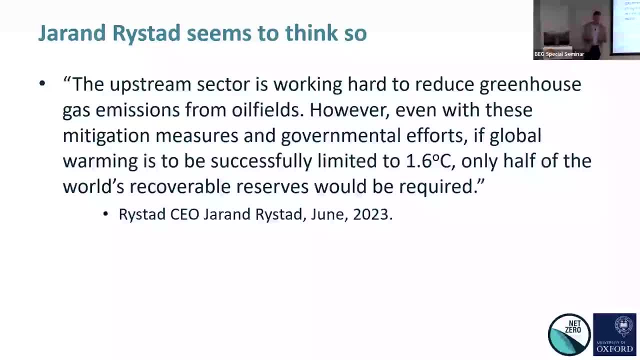 And that they, if they, that they're reluctant to invest in this industry because they think there's something hanging over it. there's this policy risk hanging over it, And of course you know there are people out there I mean, this is not Jared Reistad. 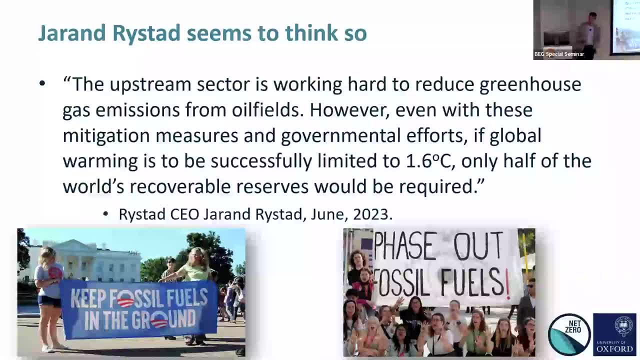 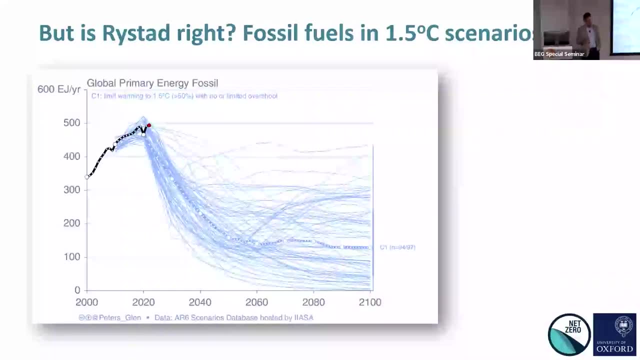 This, of course, is the people who are campaigning at COP 28 and before to say: you know, we've got to phase out fossil fuels, We've got to keep the carbon in the ground. The difficulty is that if you actually look at the scenarios that meet the goals of the Paris Climate Agreement that limit warming to 1.5 degrees, this is what happens to global fossil fuel energy use. 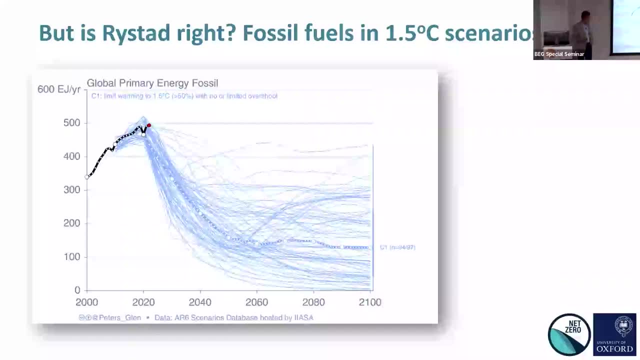 Primary energy supply. This is what happens to global fossil fuel energy use, Primary energy supply From fossil fuels. in those scenarios, Now it's a big spaghetti diagram. OK, they're all over the place, but the heavy line shows the median. 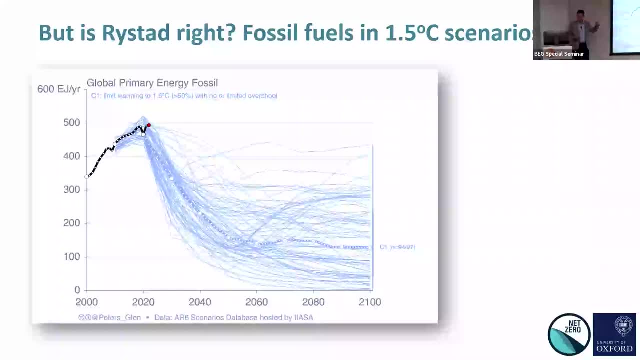 So 50 percent above, 50 percent below that heavy line, And you can see well, first of all, in none of the scenarios do we actually get to phasing out fossil fuels entirely, even by 2100.. And in the vast majority we're still using fossil fuels pretty extensively after mid-century. 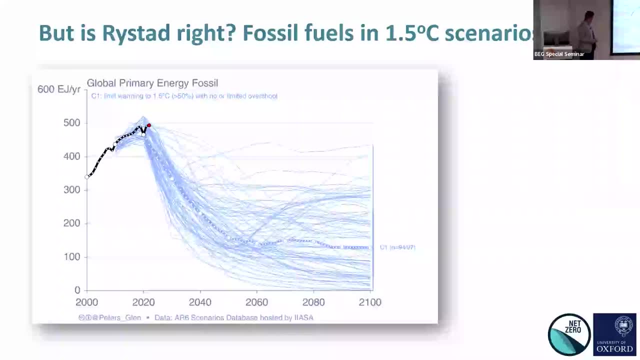 And Remember that stopping distance analogy We've stopped. I want to use my Yes. I can You know we've stopped climate change by 2060 in these scenarios And yet we're still. in the vast majority of these scenarios we're still using fossil fuels very, at a very extensive level. 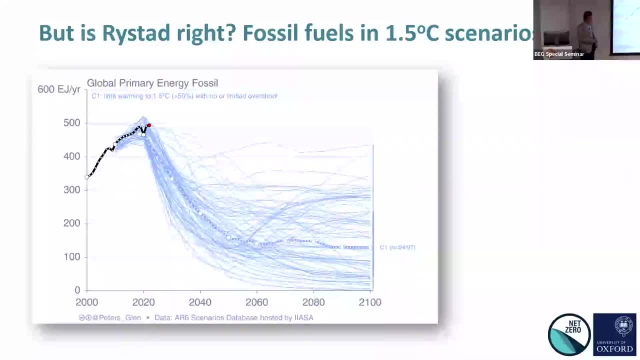 Not as not as much as we're using at the moment A couple of rather odd scenarios where we seem to keep going. I'm not quite sure what happens in those. These are: these are models of the world economy that are used to generate these. 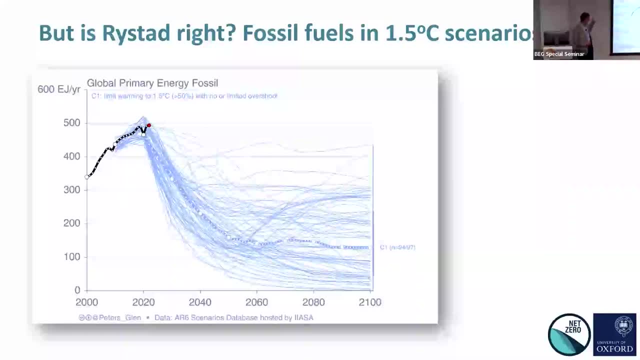 Things and they're full of loads of assumptions that are all contestable, But they give you an idea of what is feasible And it suggests that you know, as Sultan Al-Jabbar pointed out at COP. you know there is no science out there, or he was corrected himself. 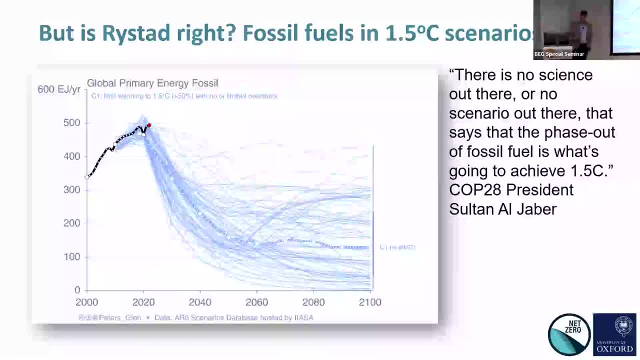 There is no scenario out there that says the phase out of fossil fuels is what's going to achieve one point five degrees. This, of course, was picked up on rather sloppily- Sloppily, In my view- by the Guardian, who said: COP president says there's no science behind demands for phase out of fossil fuels. 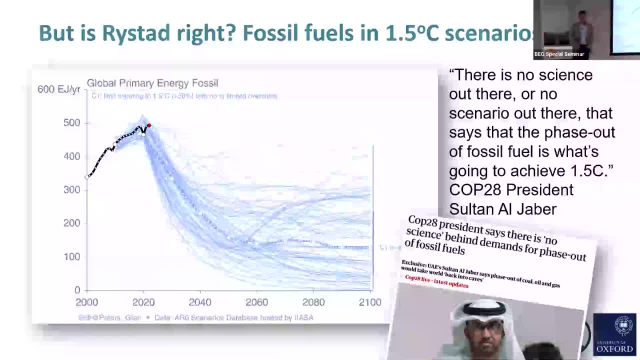 If you look carefully at what he said, that wasn't what he said. He was actually quite careful to say it was no scenario And what he said was absolutely accurate And, rather depressingly, everybody at COP piled onto him to say how he was, you know, back in the Stone Age and not understanding climate science. 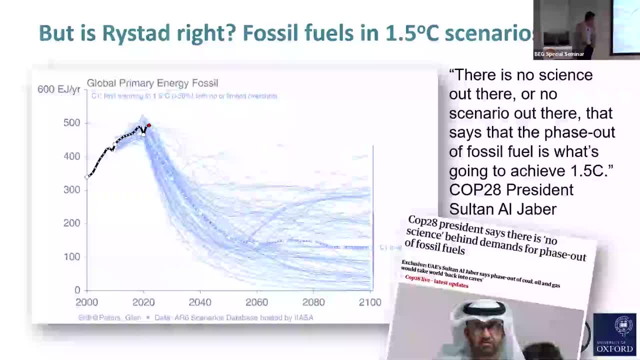 No, he was quite correct, I was. I was: Yeah, If you're on, If you follow COP on Twitter. I was one of the few people who pointed this out at the time And my comments then went completely viral And, anyway, it all went horribly wrong. 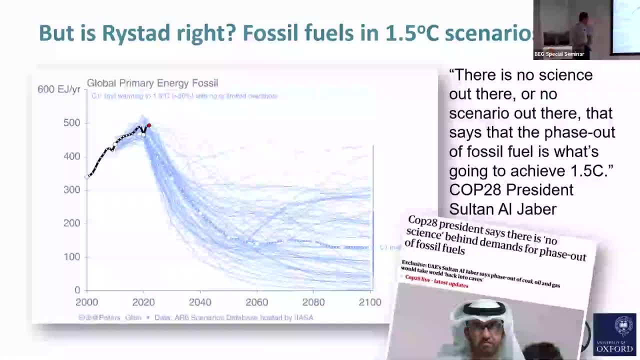 But such as Twitter for you. But it is depressing that this fossil phase out became a lot of people telling me at COP. Yeah, we know, We know about those scenarios, But the message has to be fossil phase out. I was like 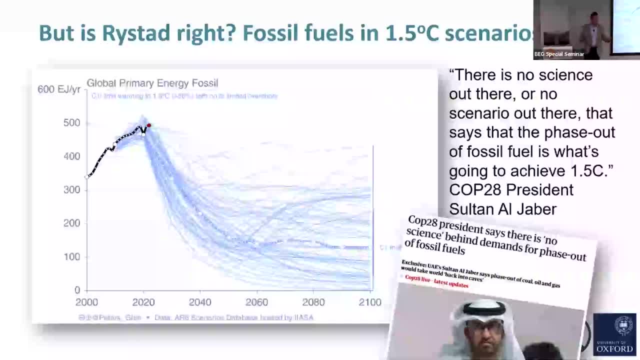 What I mean. the point is, you know, we're scientists. We're not about being on message, We're about telling people what the evidence is telling us and what our models are showing, and so on. And I do think there's a real problem in the scientists who are most engaged with the policy realm. 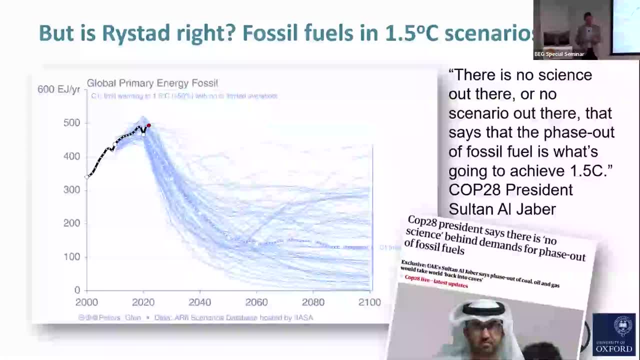 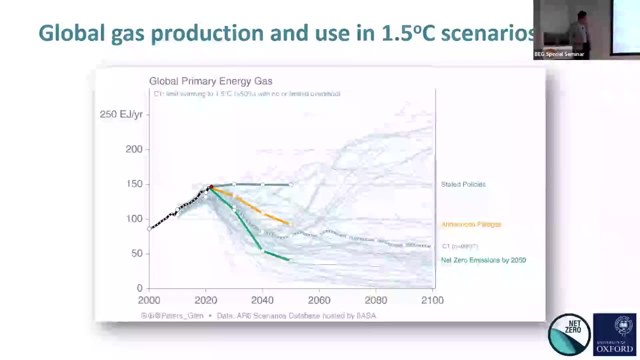 It's difficult to keep to just to the science. You get sort of dragged into to being helpful And I think we need to be careful. And I think we need to be careful about about sort of selectively sending our messages to support particular positions because if we look in particular at different constituents behind this continued fossil fuel use, this is global gas production in those one point. 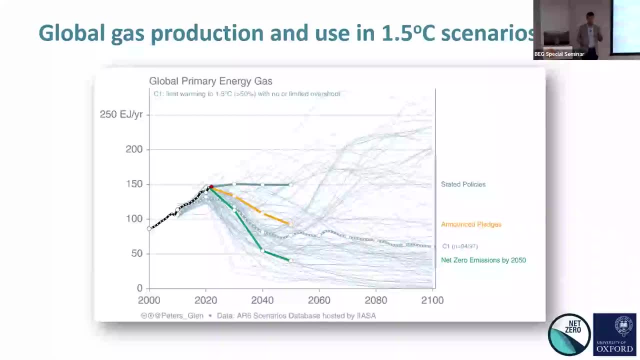 All of these scenarios meet the goals of the Paris Climate Agreement. They limit warming to 1.5 degrees And at the moment, according to BP, we have about 50 years of Of gas reserves at current rates of production globally. So that's what 50 years of reserves look like if you just assume a linear decline. 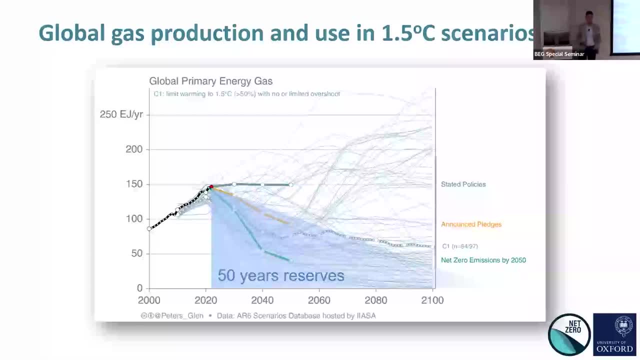 So you know, looking at that figure, it's not at all obvious that half what what Reichstadt said was that half the world's oil and gas reserves would, would have to stay underground. Well, that's not obvious from this figure whatsoever. 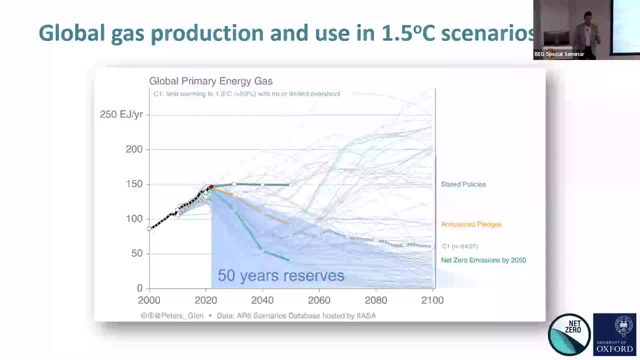 People. you know people get very upset when I point This out, but but this is what the numbers say, So you need to, you know, come up with, you know, a reason for rejecting these numbers, because you know they are the best evidence we have available oil. 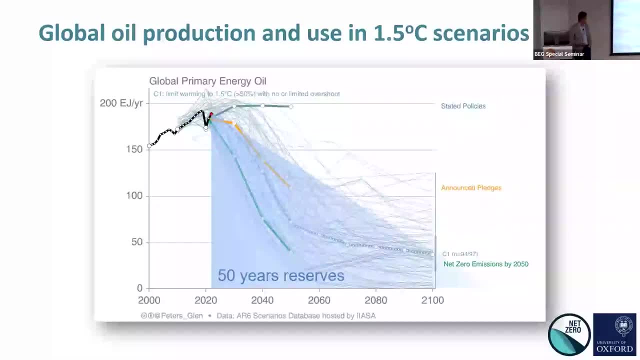 Perhaps you could argue that for oil we have too many, as it were, too much oil reserves and and this sort of, because in these scenarios we do decarbonize transport Very Rapidly. there may not therefore be the long term demand for oil that's consistent with current reserves, but there's plenty of scenarios there in which we do continue using oil later on in the century. 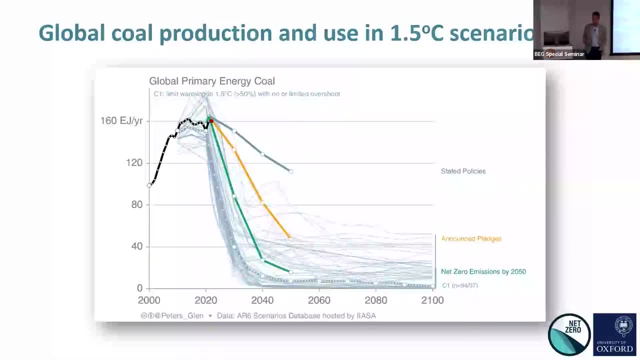 Of course, the one which is definitely stranded is coal. Coal reserves are hundreds of years of production at the current rates and we just really have to stop using coal. But there's there's many reasons to stop using coal, not just the climate one. 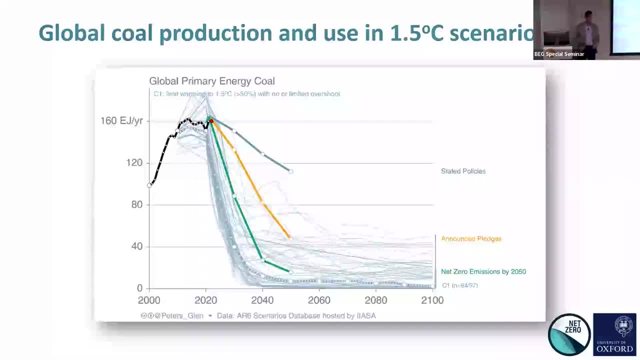 So I'm not going to pretend to you that it's all fine for every aspect of the fossil fuel industry, But I do think we need to be careful about the sort of phase out narrative applied to all fossil fuels, because, yes, we need to phase out coal. 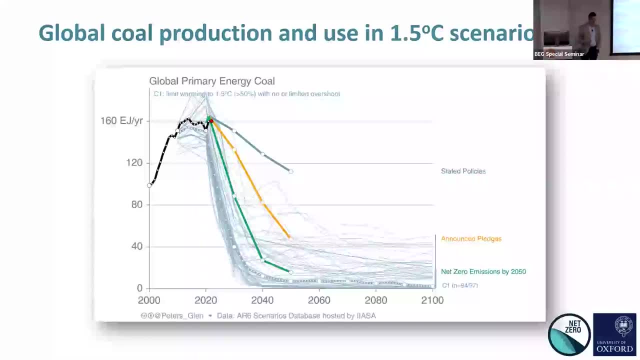 And the. although the COP couldn't quite bring itself to say phase out coal, they said phase out of unabated coal, But at least the fact that coal needs to move faster has been acknowledged. But the situation on oil and gas is that we need to fix it before we phase it out. 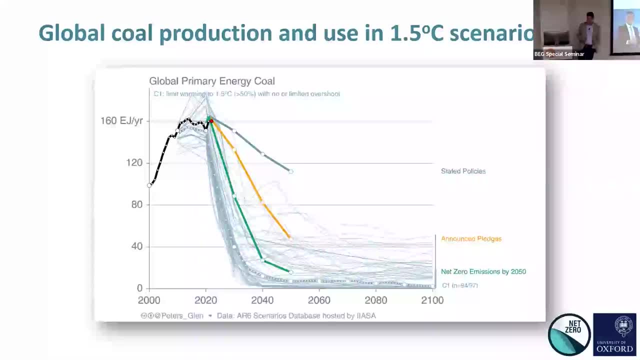 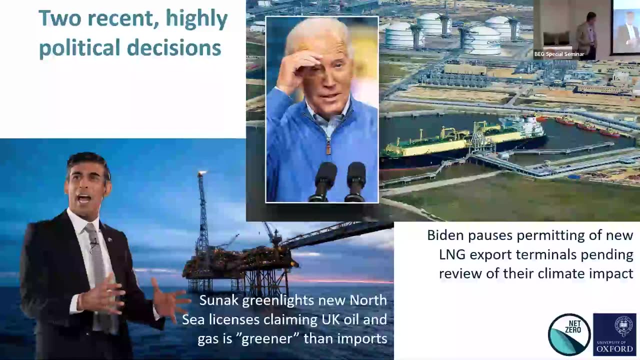 And that's what I want to talk about today. We're seeing this is starting to get very political. So in the UK, Rishi Sunak has greenlighted new North Sea licensing, claiming- and the argument they made for really encouraging new licenses of production of oil and gas in the North Sea was that oil and gas are not going to be used. 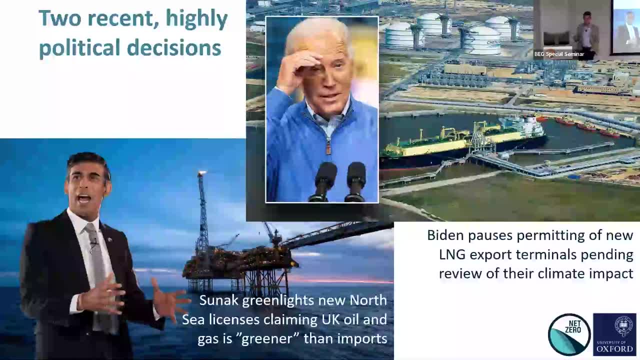 Rishi Sunak has greenlighted new North Sea licensing, claiming- and the argument they made for really encouraging new licenses of production of oil and gas in the North Sea was that oil and gas is greener than the stuff we import. So apparently, apparently UK production is greener than LNG imported from Texas. 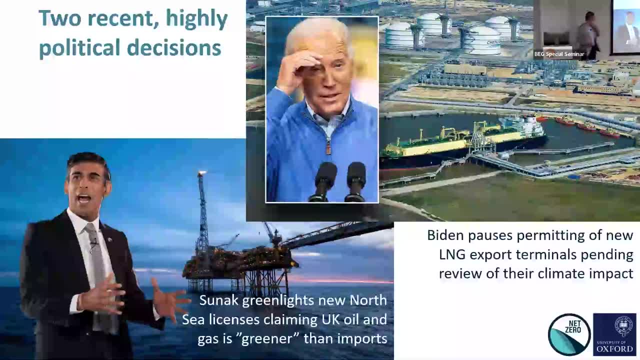 I don't know if this is true, but I mean this is the claim, And so he uses that argument to justify new oil and gas licenses. This has become political because the Labour Party, our opposition in the UK, is committed to not renewing. 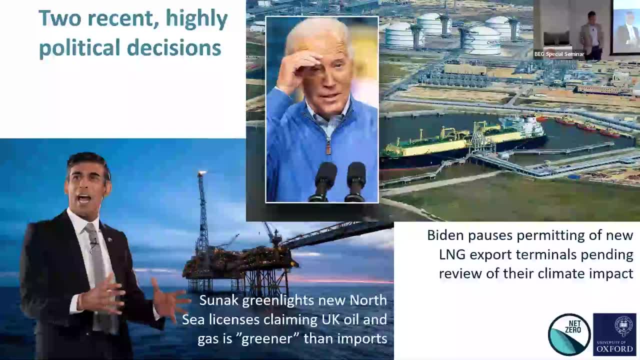 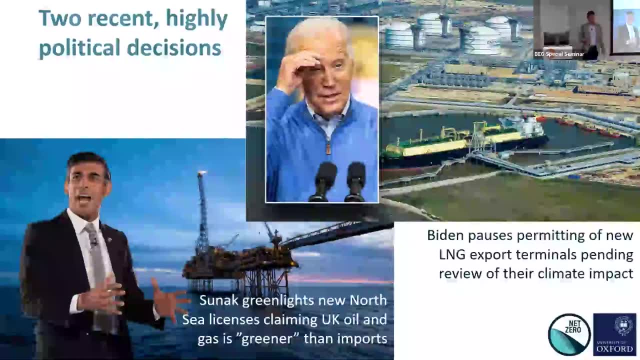 To banning all new extraction, all new licensing of fossil fuels in the North Sea, And this is therefore for the first time. climate has now become a political issue in the UK And the Conservative Party is using it to hit the Labour Party. 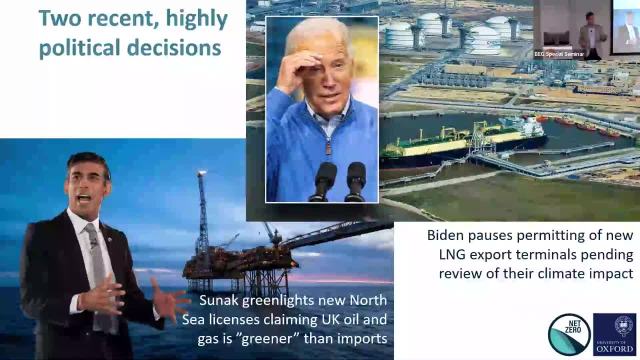 It probably won't be enough, because they've managed to hit themselves so much that it doesn't really matter what they do to the Labour Party. But who knows, We do have a relation coming up and we'll see what happens. Just in the past couple of days, we've got news that your administration 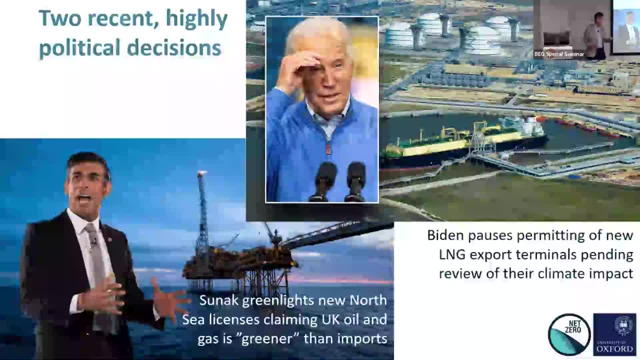 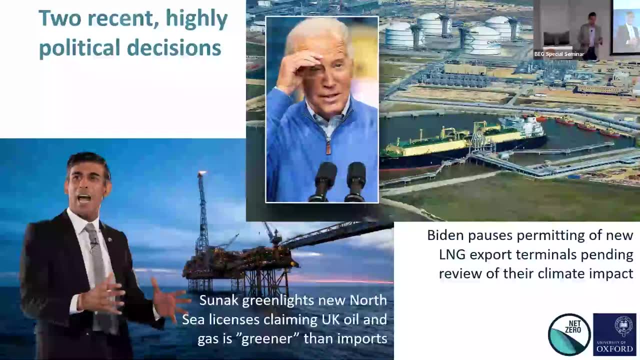 your administration here has paused permitting of new LNG exports And this has triggered a lot of discussion. And it's quite a nuanced conversation, because one of the problems with blocking it's a pause, it's not a block, but if it turns into a block on LNG exports, 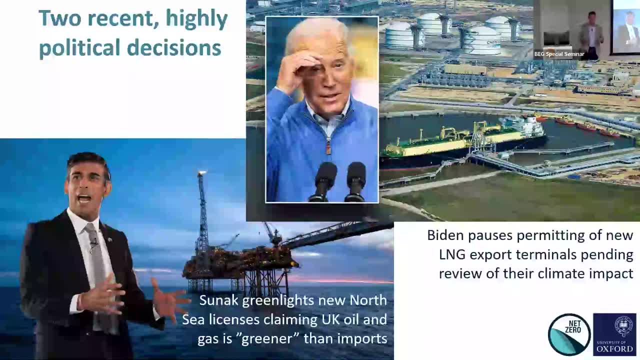 the counterfactual of what happens- and I was reading, actually, as a professor in the University of Austin has been commenting on this in the press recently. the counterfactual of what do countries use instead of LNG imported from the US is really important to determine whether or not that actually has a beneficial impact on global climate. 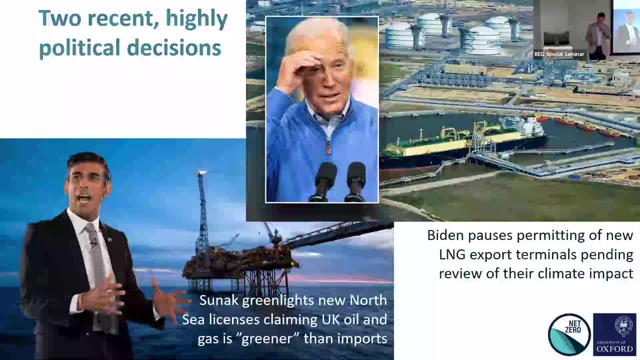 So you know it's. these are. these are both both the Labour Party's position saying no new oil and gas extraction in the North Sea and the Biden administration's position saying, potentially possibly saying, no new LNG export infrastructure in the US. They're quite vulnerable decisions because they don't obviously deliver on the climate objective. 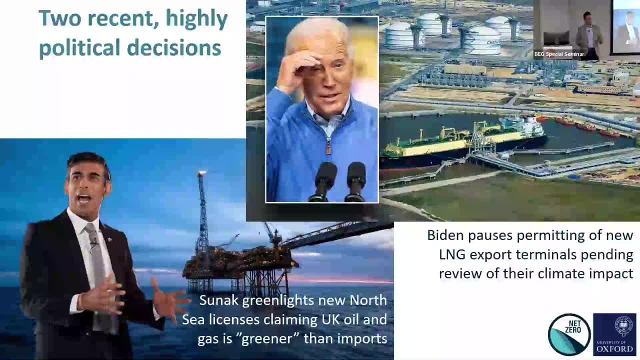 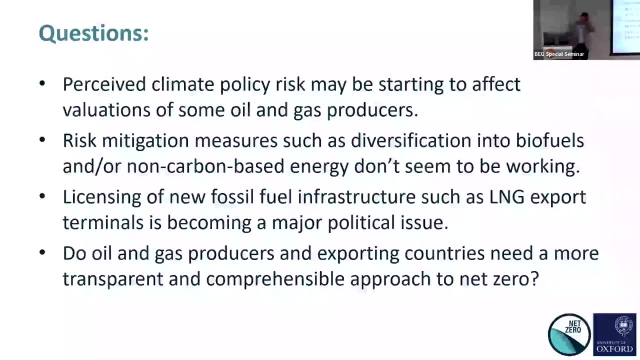 They sound like they sound good to environmental activists, But are they actually coherent policies? And and if you have an incoherent policy, it's much more vulnerable, obviously, to the to the other side to criticize It. So you know, this is the questions we'd like to sort of address here. 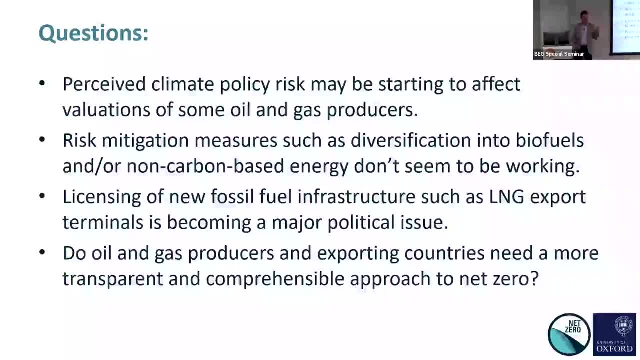 We've got this interesting sort of undervaluation problem of oil and gas companies And, and in particular, in Europe. this is probably more relevant in Europe, But our European oil and gas companies are talking a lot about how they're diversifying themselves into general energy companies. 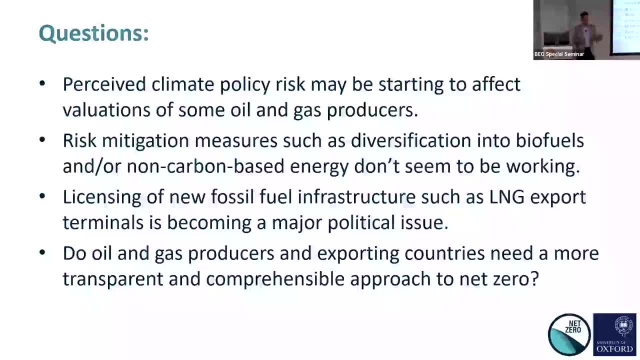 And they're and they're investing heavily in biofuels and nature based solutions And so on, But it doesn't seem to be working. The market doesn't seem to be impressed at all And, in fact, in many ways, the market is rewarding US oil and gas companies who have a very clear climate strategy, which is like whatever. 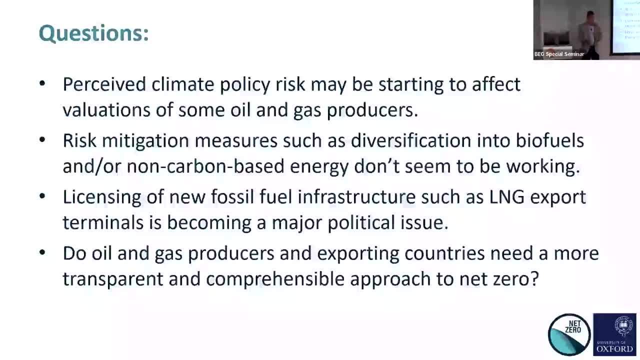 I mean that seems to be. the market seems to be quite comfortable with a very clear strategy, even though the strategy is not really a strategy, but at least it's very clear what it is, And so so. so this sort of confusion Over what the oil and gas industry is going to do is actually starting to perhaps potentially cost the industry itself. 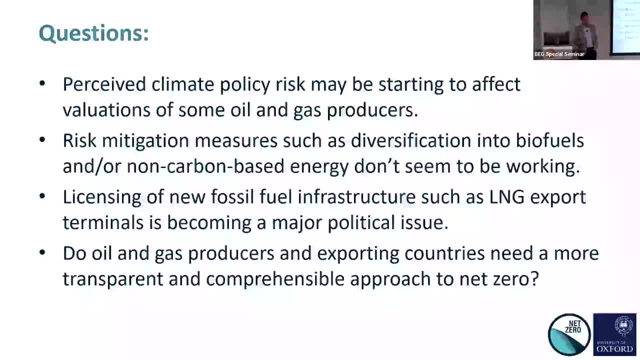 We also have confusion over licensing governments involved, involvement in licensing of new infrastructure, because you know these arguments about is it? is it needed? Is it helping, As it actually is banning it going to help? or just move production to different parts of the world? 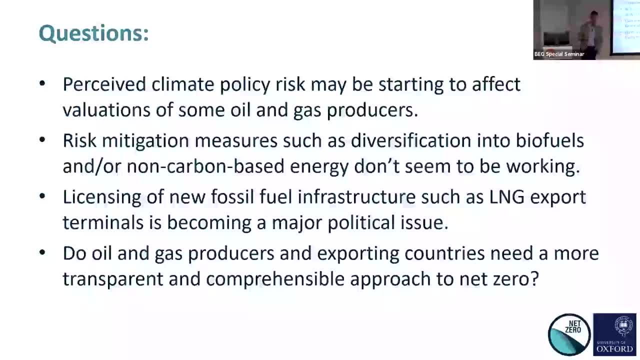 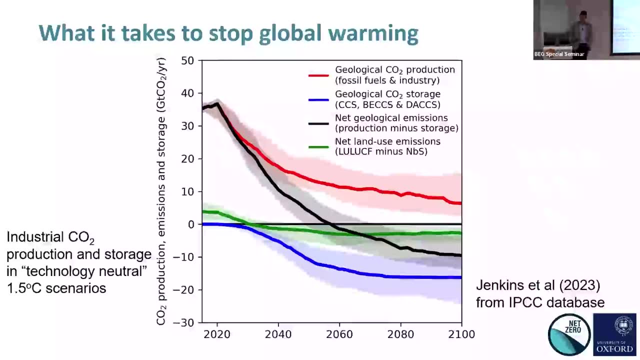 So question to us: do oil and gas producers and exporting countries, or exporting states like the state of Texas, need a more transparent and comprehensible approach to net zero? And that's what I want to talk to you about. Just to get back to basics, this is what it takes to stop global warming. So these are those scenarios. 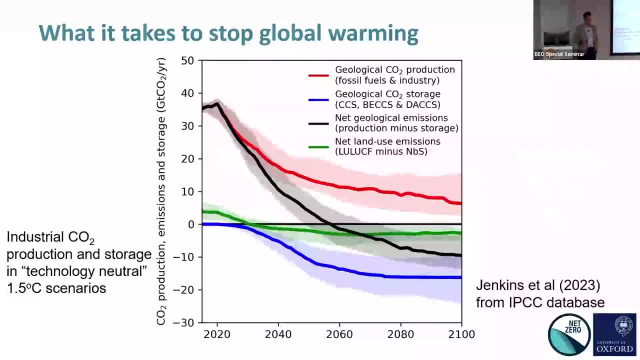 that I showed you earlier that meet the goals of the Paris Climate Agreement. And I've got rid of the spaghetti by just showing you the median pathway and the 25 to 95, 25 to 75 range. So it's an indication of the range And in red it's carbon dioxide production from fossil 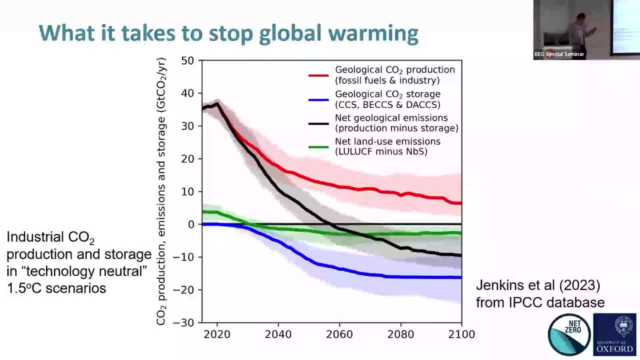 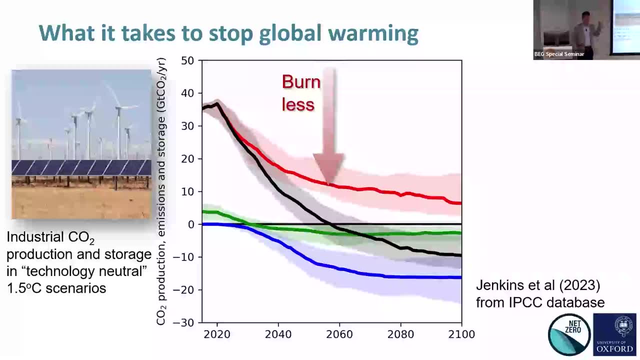 fuels and industry. So, as you can see, that goes down. We do produce, we burn less by replacing production with solar, And this is what everybody knows about. This is all happening, But it's not. It doesn't go remotely close to zero. It goes down by maybe 75% And then we achieve net zero. 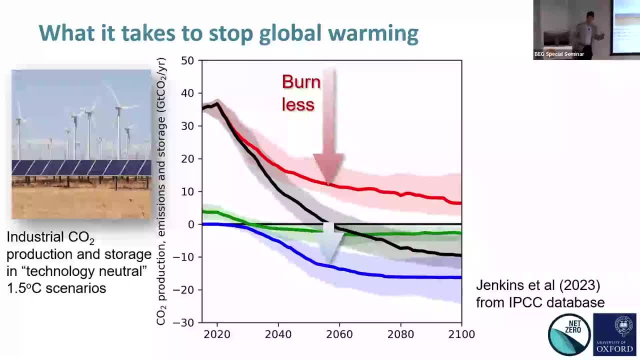 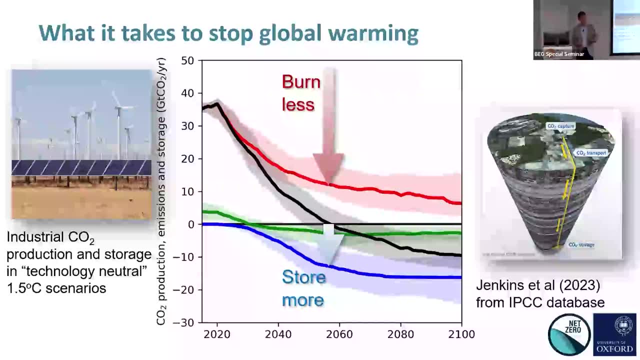 by storing a great deal more. And the blue line there is the carbon dioxide we store back underground. So this is currently 40 million tons of carbon dioxide per year re-injected back underground, And it goes up to somewhere between 10 and 20 billion tons of carbon dioxide per year. 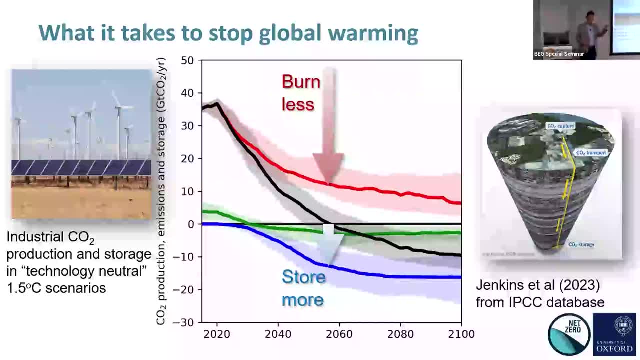 by mid-century And the scale of that transition. this multi-hundredfold increase, so going from 40 million to over 10 billion, is a factor of 250. increase in the rate at which we inject carbon dioxide back into the Earth's surface is overwhelmingly the biggest challenge in dealing 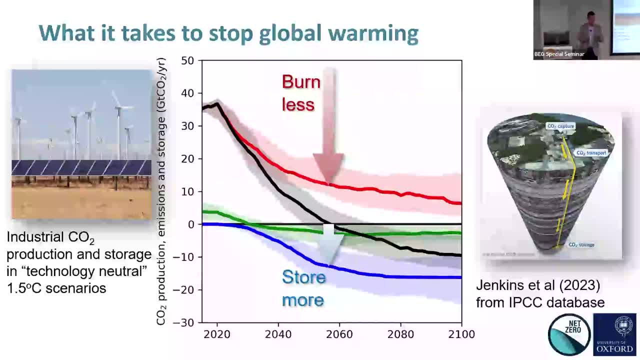 with the climate issue. You should be honored that you have people like Catherine here working on solving that challenge, But unfortunately there's only one of her, or at least not very many of her, And that's a real problem we've got at the moment because if we look at- sorry, I digress on something else, but 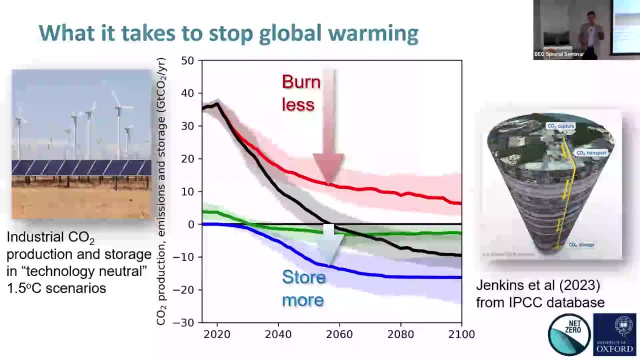 we'll come back to that. But the scale of that challenge is so huge and so badly underestimated and completely downplayed by the fossil phase-out argument which is: oh, we don't need to store fossils, We don't need to store CO2, because we're just going to stop using fossil fuels entirely. 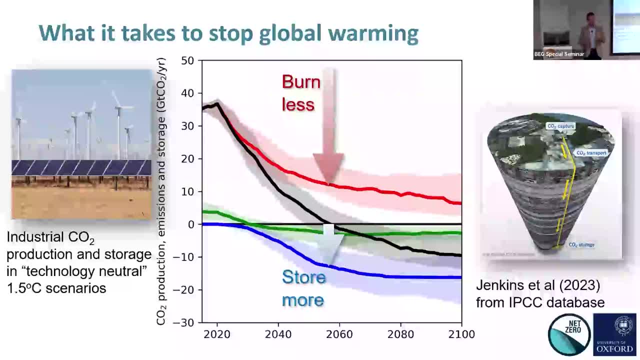 Well, the answer is we're not And therefore, neglecting our obligation to drive up carbon dioxide storage is absolutely essential. There's a green line here which I will want to talk about, which I want to talk about because it's become in my 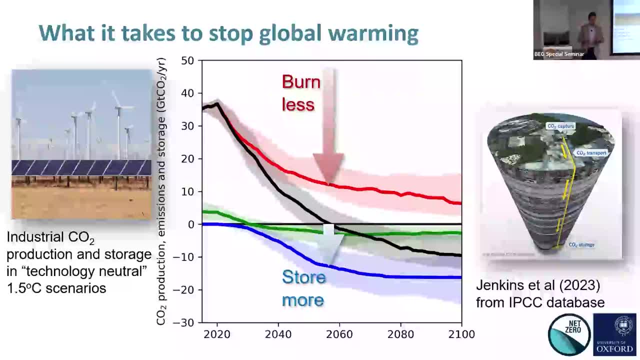 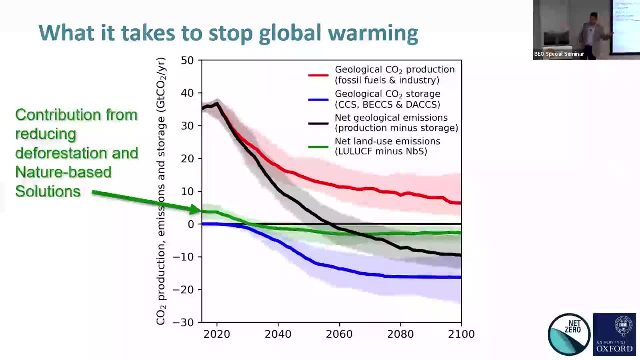 view a bit of a distraction in the big picture here, But I'm going to digress a little bit to address it. And this is the contribution from reducing deforestation and the transition to nature-based solutions to remove carbon dioxide from the atmosphere. 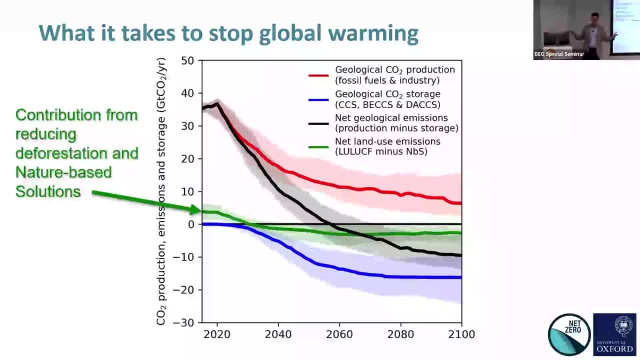 This was massively talked about at COP28.. It's always talked about heavily at COPs. Everybody loves to talk about it. Planting trees, restoring mangroves, restoring coastal ecosystems to absorb carbon and, obviously, reducing deforestation: They're all great things to do and they do provide some contribution to achieving net zero. 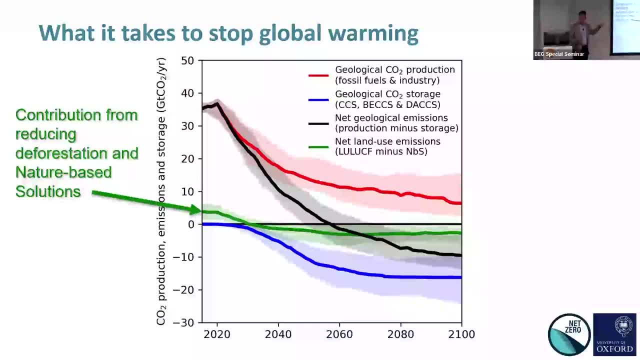 But you know, do look at the lines here- That green line is quite close to the zero line. If it wasn't there, it wouldn't really change the big picture very much, And so it is important to keep that contribution from nature-based solutions into perspective. 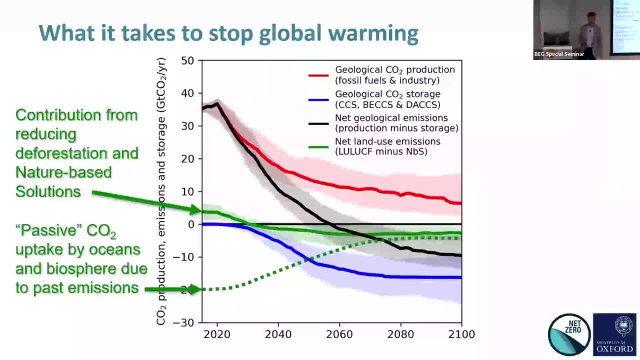 There's also a real problem that we are facing at the moment, which is that you know we're not going to be able to do anything about it, But this is not the only carbon that's being absorbed by nature over the next few decades. 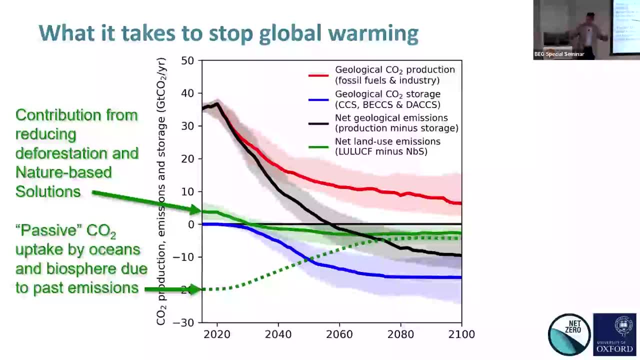 because nature, the biosphere and oceans are absorbing carbon at a massive rate already just because of past emissions, because we've driven up carbon dioxide concentrations in the atmosphere. the biosphere is responding, the oceans are responding and taking up CO2.. 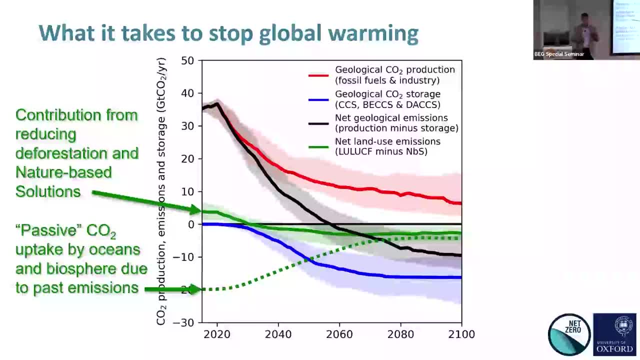 So actually distinguishing between carbon dioxide we deliberately put back into the biosphere and carbon dioxide that's being taken up by the biosphere anyway, just because of the way it's responding to past and present. climate change is virtually impossible And because of this it's a small contribution and also a source of considerable confusion. 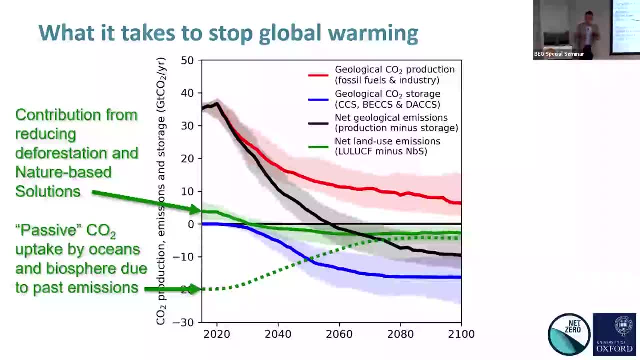 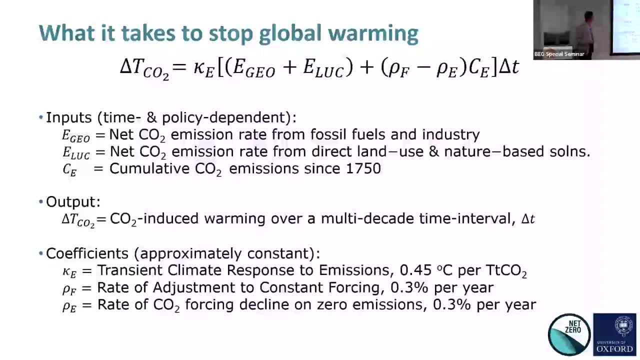 and actually is really holding back, focusing on what we really need to do at the moment. I was going to show you an equation of this. Well, I'm going to show you an equation because you know, hey, I do come from a physics background. 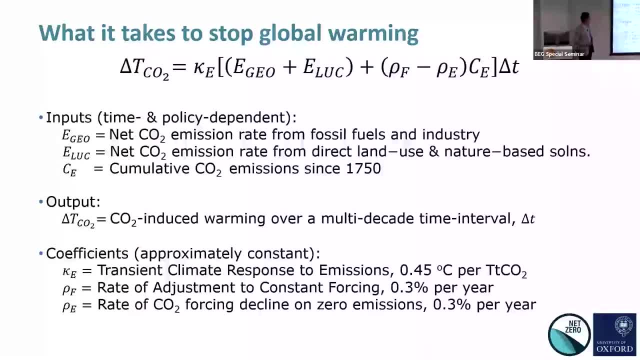 so it's an important equation because it tells you what drives carbon dioxide induced warming. And it, by the way, for those of you who don't do climate modeling, it's quite a useful equation because pretty much all the really complicated climate models when it comes down to their 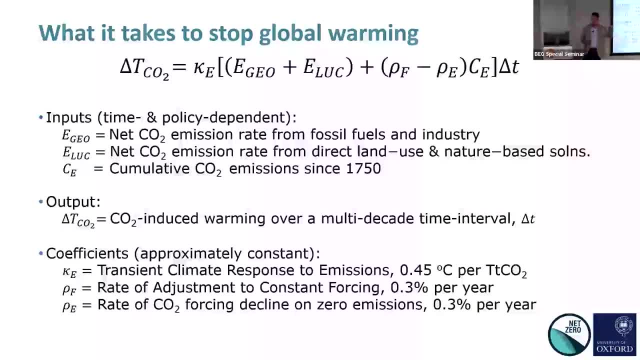 behavior in terms of global temperature. this equation is pretty much good enough. Now I noticed people who do do climate modeling are looking at me suspiciously here saying: Are you going to do that because of the forehead instrumental taught really to you to change the world temperature drive? 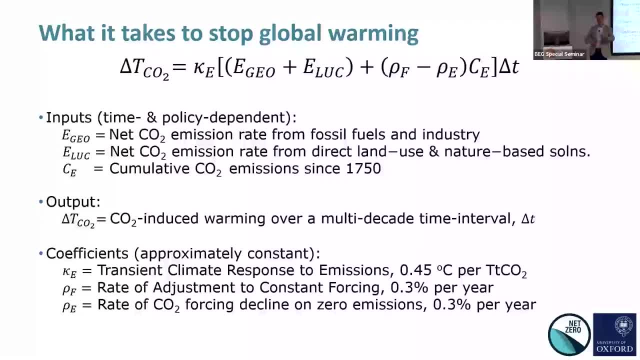 Ну, bias, I don't mean I'm going to control the climate, Of course, by sort of ridiculing our entire profession. Of course, all this tells you is the implications of emissions for global temperature. It doesn't tell you anything about the weather. It doesn't tell you anything about the oceans. 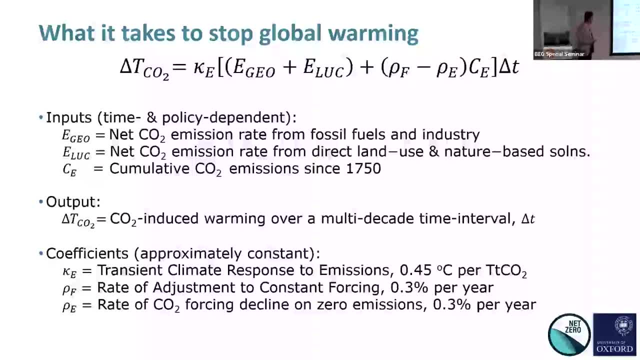 it doesn't tell you anything out anything else, But it does tell you how emissions at the moment and in scenarios that meet the Rhodes of the Paris agreement relates to global temperature. So it's worth going through. These are two contributions, Two contributions here. 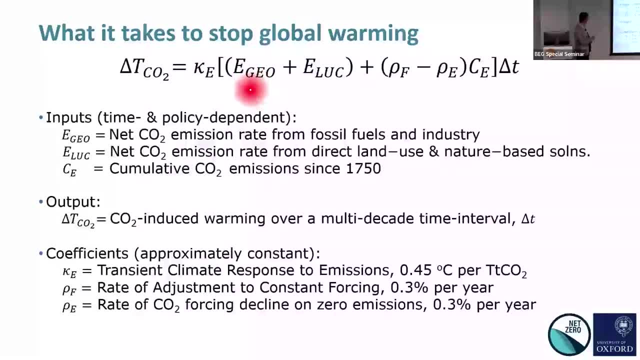 One from geological origin- carbon dioxide- and land use- carbon dioxide from active land use change. So deforestation or deliberate reforestation, So active interventions in the biosphere. That's not the passive removal, that happens because climate has changed anyway. And then over here- So people kind of know about this bit- You put more CO2 into the atmosphere. 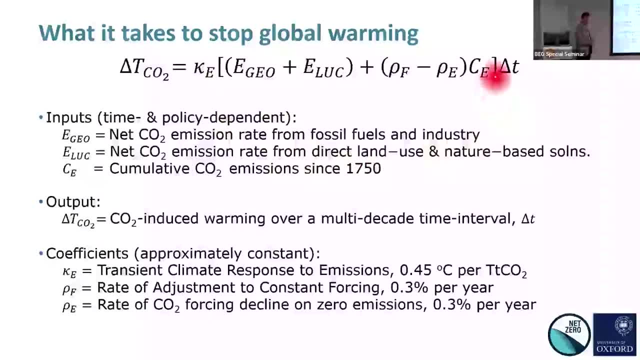 You multiply by constant and the length of time you do it and you end up with the warming. So that's the sort of cumulative impact of carbon dioxide emissions on climate that's been well known for decades Over here. I've written in this extra term here Those two rates. 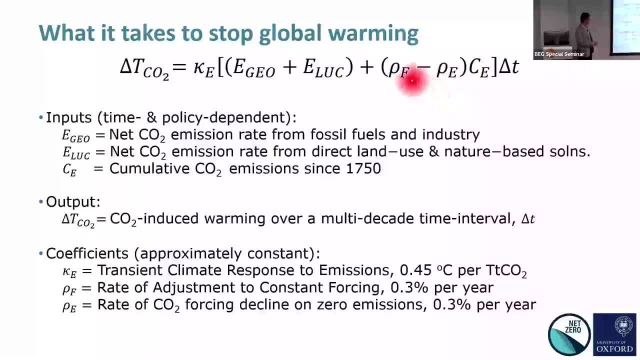 These are. these are both have units per per year. These are rates of adjustment, both the rate at which the world would warm If you were to freeze atmospheric CO2 concentrations. So if you were to stop concentrations from rising today, but not reduce them at all, just keep them steady, then the world would continue to warm and it would continue to warm at a rate of roughly 0.3 percent per year, 3,, 3 percent, 3 percent per decade. 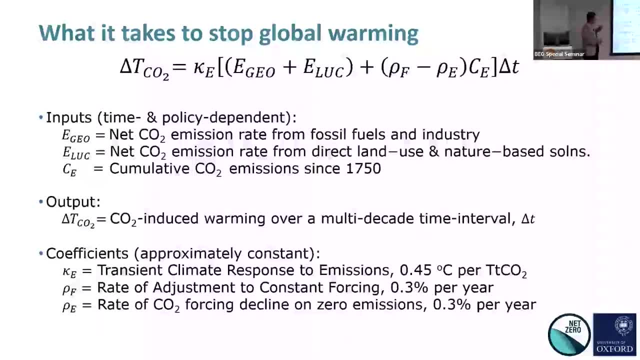 So that's that term, But. but if we Reduce emissions all the way to zero, then there is a. The natural carbon cycle takes carbon dioxide back out of the atmosphere. reduces carbon dioxide concentration in the atmosphere just fast enough to balance this rate of warming. 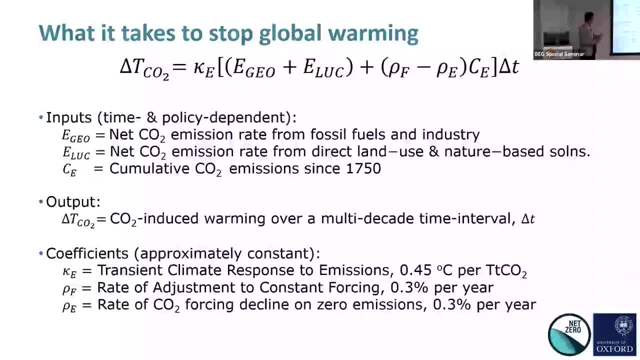 So we end up with these two rates which cancel, And you have this passive carbon dioxide removal by the biosphere notions, which is really important. It's equivalent to active removal of 10 billion tons Of carbon dioxide per year By mid century, in a one and a half to two degree scenario. 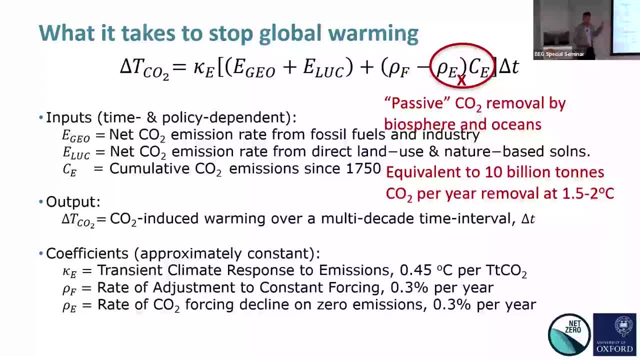 So this is, this is not a small term. I, I'm, I'm stressing: they cancel, So they add up to zero, but neither is small. Yeah, the warming after the ongoing warming, after CO2 stabilization, would add up to about half a degree per century. if that's all we did, 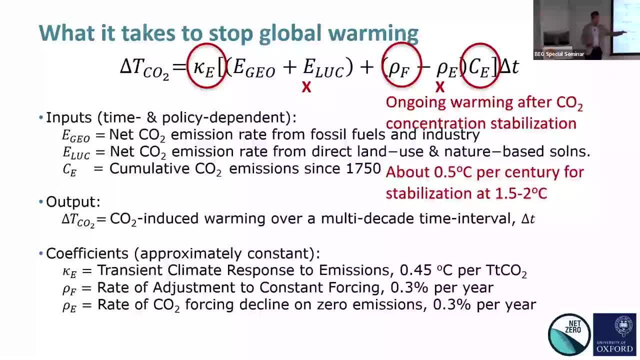 So we do need the biosphere to be taking this carbon out of the atmosphere. We also We need to protect the biosphere in order for it to be doing that, But we can't regard that as part of this land use change emissions. 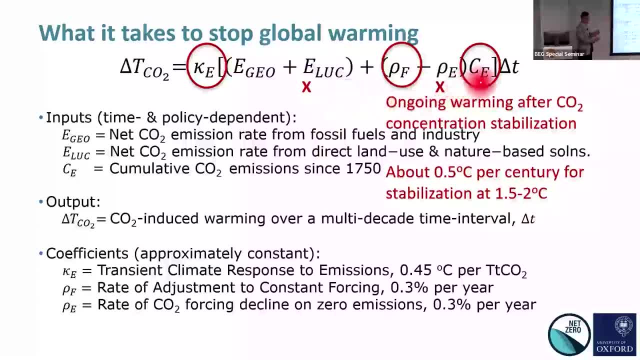 If we, if we muddle up this passive removal of carbon due to past emissions with our active removal by planting trees or or restoring mangroves, then potentially we double count the same carbon removal. We take credit for carbon Removal. That's happening. 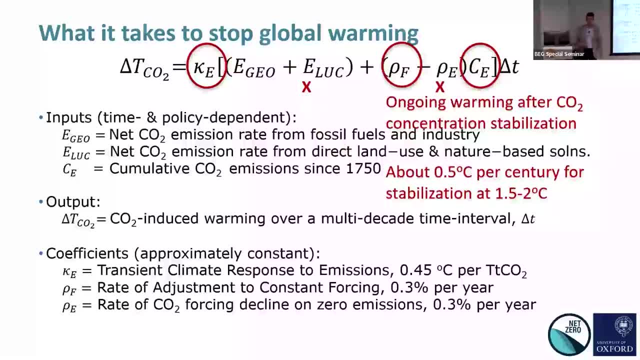 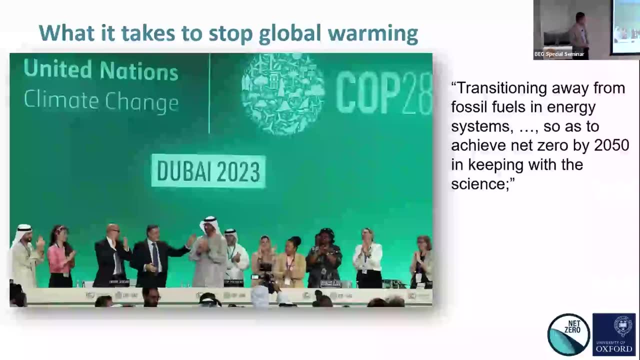 We're doing it anyway And use it to offset our ongoing fossil fuel emissions, And if we do that, then we don't end up with we don't end up stopping global warming at all. And this is an issue because you know, the great headline achievement of COP was that we were going to transition away from fossil fuels and energy systems so as to achieve net zero by 2050, in keeping with the science. 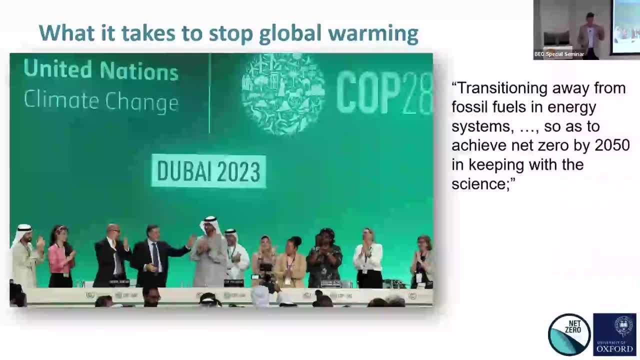 And a few of us who were there while this was being discussed, Point pointed out- and I know this was raised because I fed it into one delegation- who said, yeah, they would take it forward. Doesn't net zero need to refer to something like net zero emissions or? 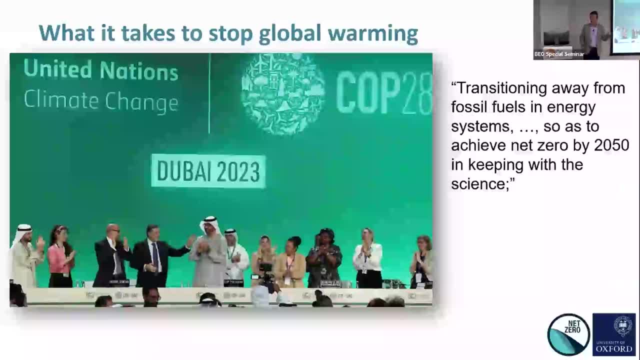 net zero something, And apparently no, we're just going to achieve net zero. Okay, So you know, okay, So obviously you know, diplomacy is the art of the art of the possible And I think actually that full credit to the UAE presidency. it was a tremendous achievement, They got this. 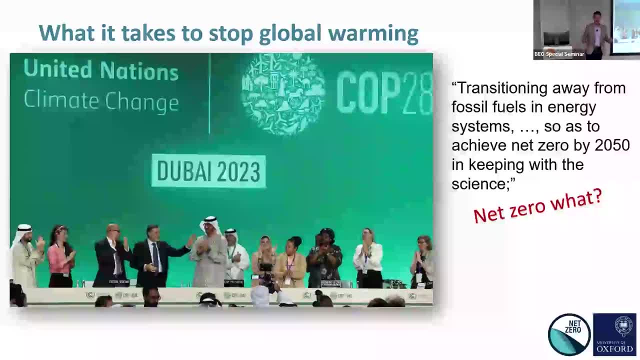 language agreed by everybody. But one of the prices of that is you just have to have phrases in there that maybe don't make a whole lot of sense. So they're aiming to achieve net zero, but they won't say exactly what net zero what. And the difficulty is, if we look at 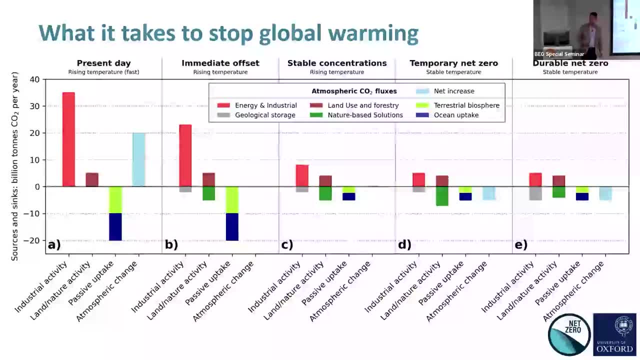 flows of carbon into or out of the atmosphere under different scenarios. so the left. here we have the present day, So lots of carbon being dumped into the atmosphere, quite a lot being removed by this passive response of the oceans, but not enough. So carbon concentrations are rising in. 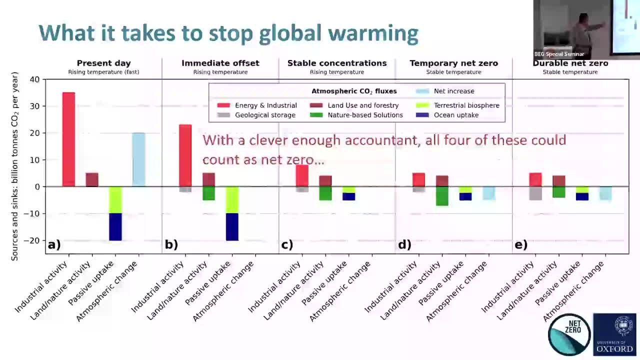 the atmosphere. That's the situation we're in. So if we were to reduce our emissions immediately by less than 50% and sort of bump up nature-based solutions and so on, we could stop concentrations rising and, on current accounting rules, claim we've achieved net zero. Of course that wouldn't. 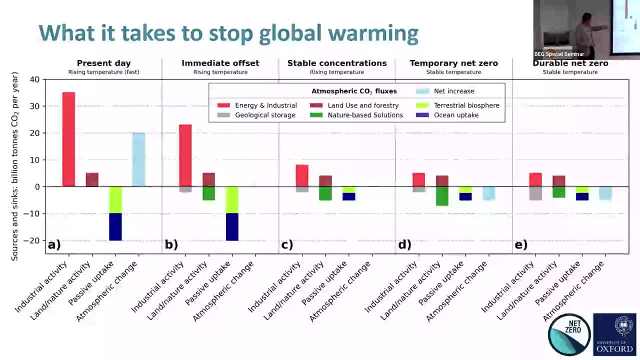 last very long, because as soon as you stop concentrations rising, the biosphere and oceans, there's the light, green and blue bars there take up carbon less rapidly, But they keep taking up carbon And so you know we're in a situation where we're in a situation where we're in a situation. 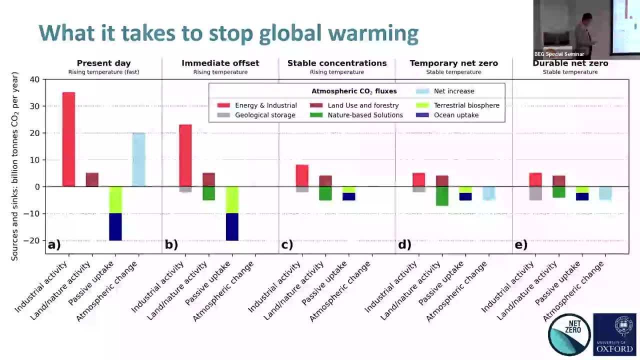 where you know we've got some answers here, But there's some other cases where we can get back to the point where we're still on the same fast track for today, to where we think that India is gonna get those next four to five years. So far we're getting strong enough to get totals. 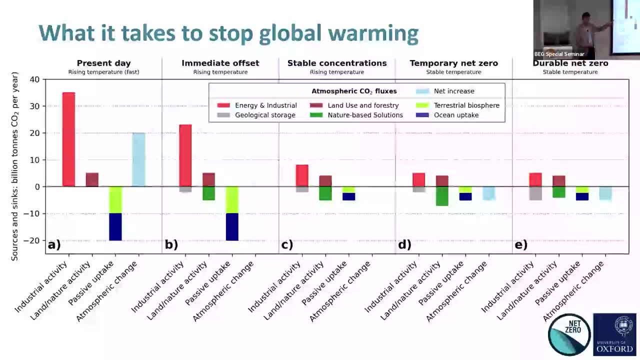 back to 10, but all of these other effects of the effects are just going off and moving at continuous speed. And so, even after a few decades, you could get to a situation with you get a situation where- And so even after a few decades, you could get to a situation with you get a situation where You 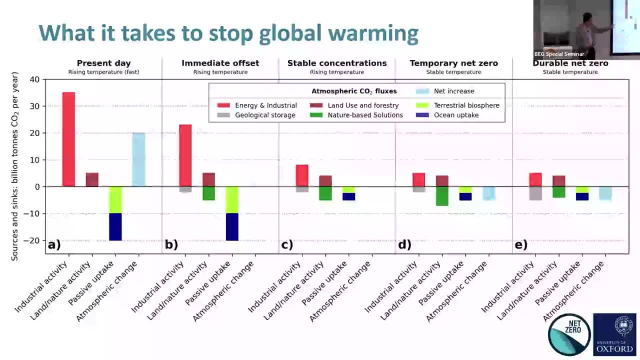 have a balance between ongoing fossil fuel use and uptake by the land and the oceans, which keeps concentration stable. but it's not enough to actually stop global warming and to stop global And we you need to get to, you know, either panel or a and sticks domesticductors also. 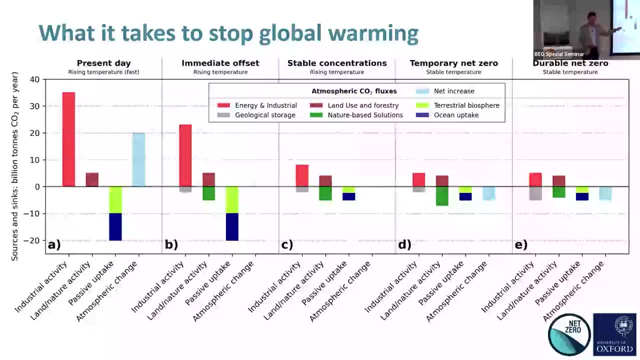 fossil fuels and storage of carbon in the biosphere. So there's some balance in the red bar and the green bar, But that can't last very long because you know there's limits to how much we can rely on the biosphere to absorb ongoing fossil fuel emissions. So we've argued in this and other 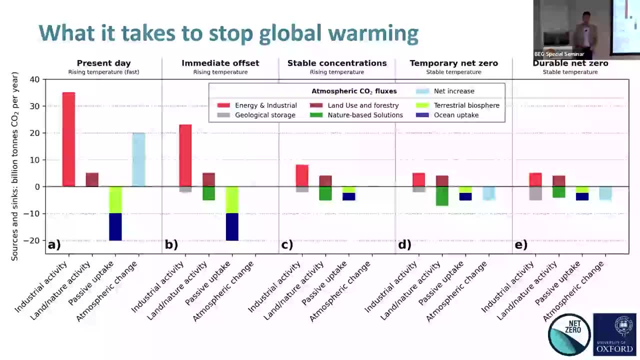 papers that the only durable net zero that would actually stop global warming- for, you know, multiple decades- is one in which you have a like-for-like balance between any continued generation of CO2 from burning of fossil fuels is balanced by geological disposal, So engineered. 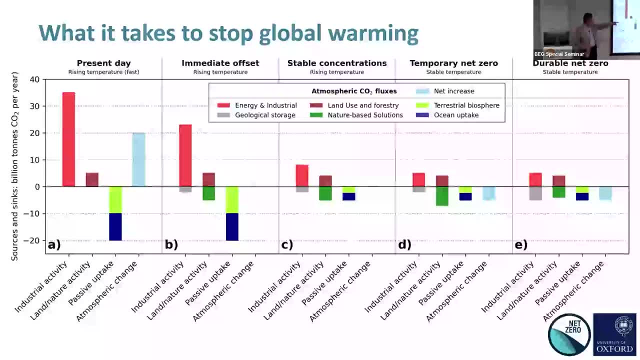 capture and re-injection back underground. So that's why there's a balance in the red and the gray bar And that if you're still producing emissions from food production, from the biosphere, that's the brown bar. you're balancing that with your nature-based solution. So the idea that 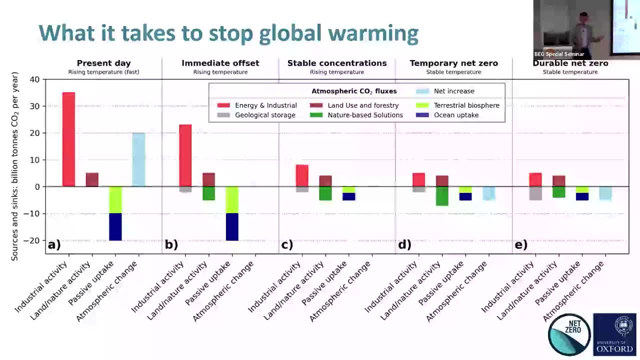 you can balance continued fossil fuel generation of CO2 with nature-based uptake is a very good idea. So I think that's a good idea. I don't understand why it makes sense to anybody, because you know you've only got to stop and 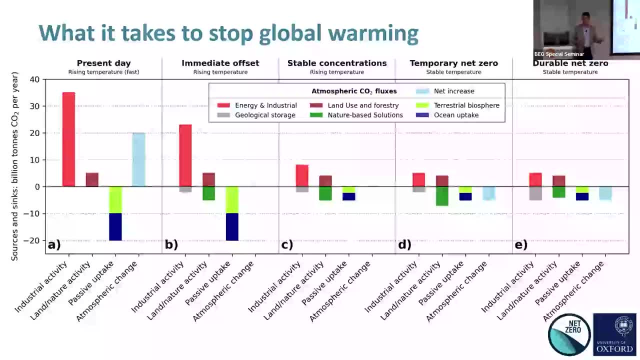 think about it. We can't turn rocks into trees forever. But there's huge enthusiasm for this because, of course, it is a much lower cost and quite attractive approach to addressing emissions at the moment, And the difficulty is that you know if you've got a good accountant all four. 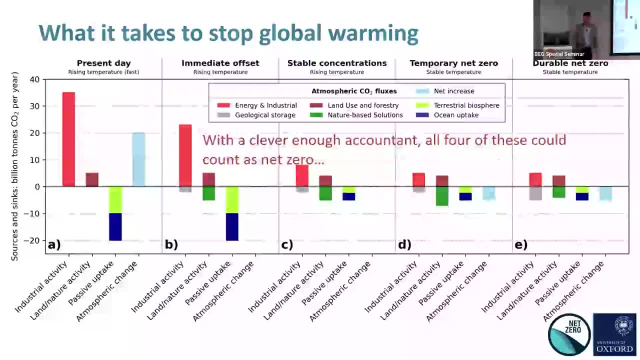 of those could count as net zero. And in fact if you're just one player in the world, you're not the world as a whole. So if you can find enough of this stuff to balance your emissions, you can claim to be net zero. 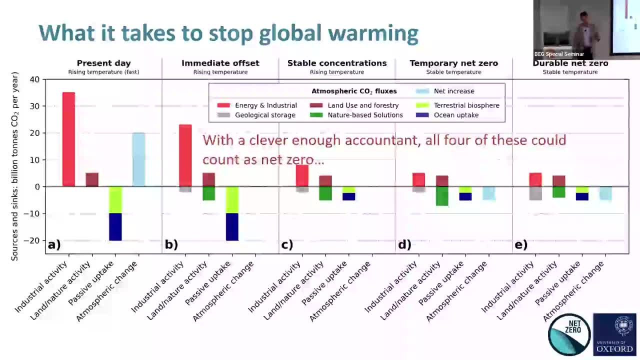 already. So if you want to, if there's graduates in the room who want to have a profitable and immediate, highly profitable job, move into the carbon credits space and start advising companies on how they can make themselves look net zero And you know you'll have a good life. Just a. 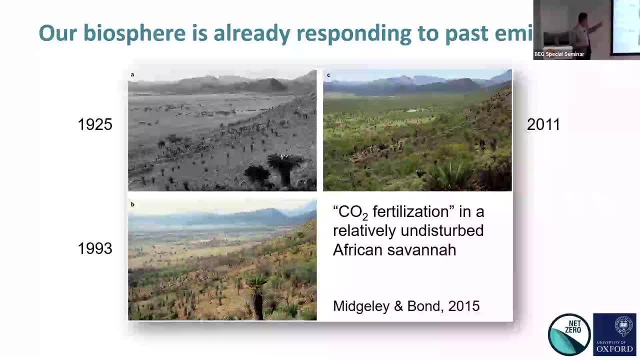 quick side note. We've had a couple of really good examples of how the biosphere has already responded to past emissions. You can see this is the same scene in Africa And you can see how the vegetation has transformed over the past century. And you know Bond and Mitchell and Bond looked at this. 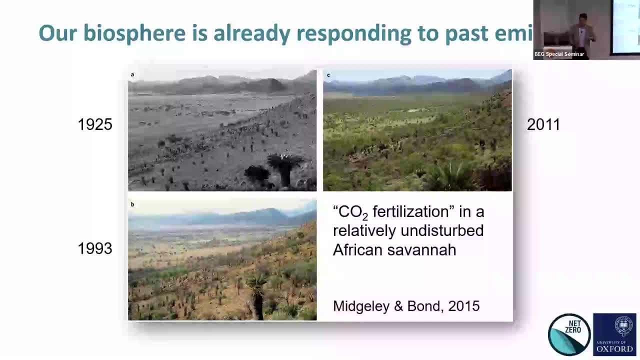 modeled it and established that that recovery of that it's not really recovery, because this is actually the biosphere moving to a new unnatural state for that part of Africa is because of the extra CO2. in the atmosphere. So this is happening And it's happening all over the world. This shows you where. 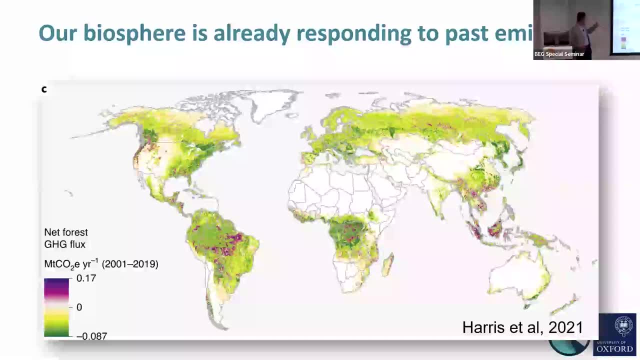 up until 2019, so before all the forest fires in Canada, although the little purple patches are where there have been forest fires over that period- we've got absorption of carbon dioxide by the biosphere And if you just add this up, Canada's forest sink over that 20-year period. 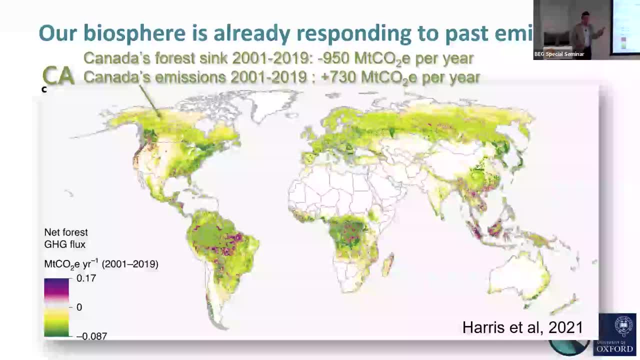 was about a billion tons of carbon dioxide per year. Canada's emissions- any Canadians in the room note- were about three quarters of a billion tons. So people in Canada have noticed this and say: wait a minute, we're net zero already. Well, I mean yes on the accounting rules used by the. 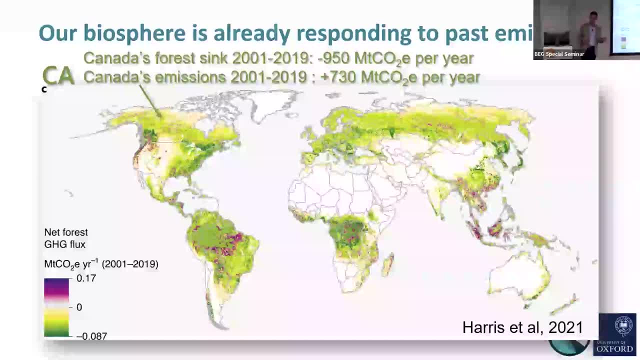 UNFCCC? they kind of could be. But that's a problem with the accounting rules Because if we all declare that, if we all take credit for the carbon dioxide emissions, we're going to have a billion tons of carbon dioxide per year. So if we all take credit for that natural response to the 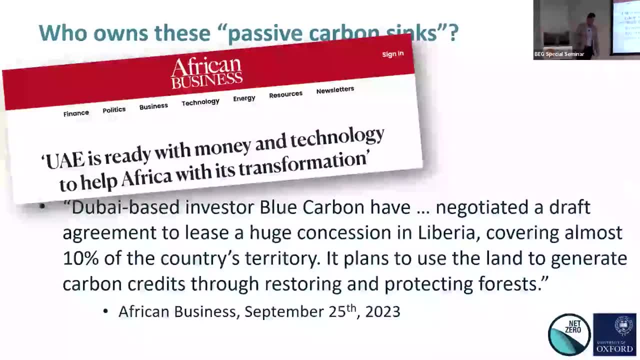 biosphere. we won't stop global warming And we're seeing this happening all over the place In the buildup to COP. we heard about a Dubai-based investor, Blue Carbon, have just leased 10% of Liberia for carbon credits, So this is turning into huge business, which will be very, very. 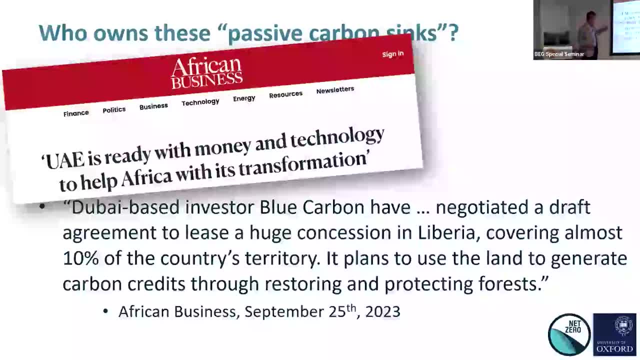 difficult to unwind Now, both Blue Carbon or Blue Carbon. you can probably afford to drop a few, because I mean, you know they're probably quite rich. But Liberia's economy is now becoming dependent on this carbon credit market, And this is a real 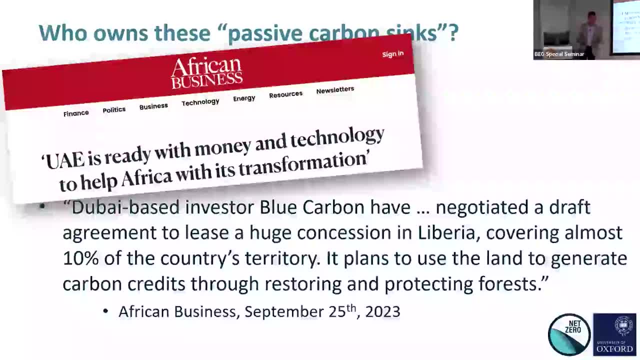 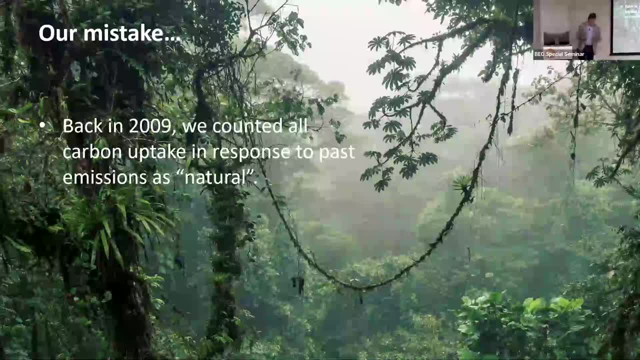 concern. So, even though I'm saying it shouldn't be a problem, I'm digressing onto it because it is a real issue at the moment And it's one I feel strongly about because, you know, when we published all these papers in 2009,, it didn't occur to us that this response of the 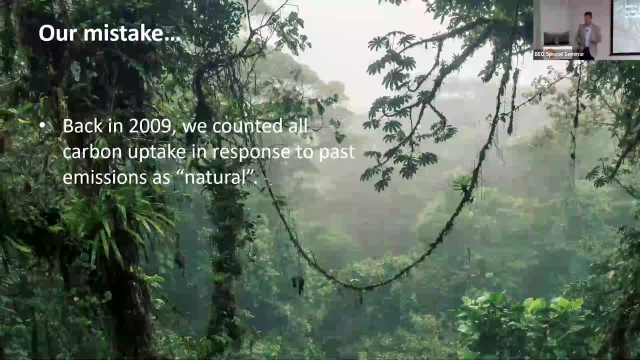 biosphere was anything other than natural. Of course it's not entirely natural, because it's happening because of our past emissions, but we called it the natural response to past emissions. We didn't call it greenhouse gas removal, But unfortunately the United Nations rules allow countries to take 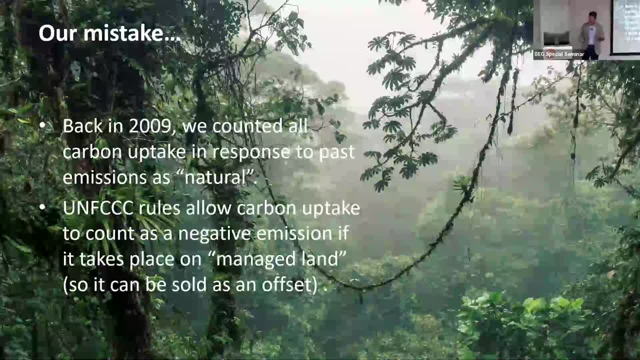 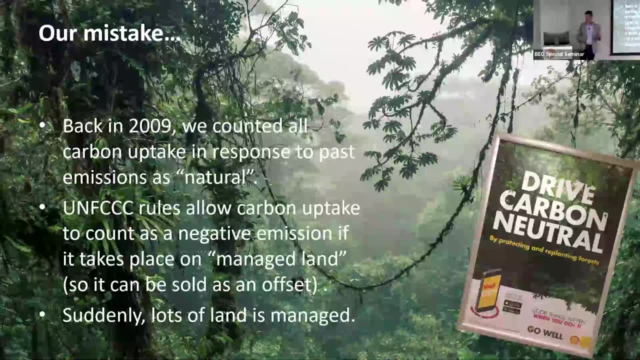 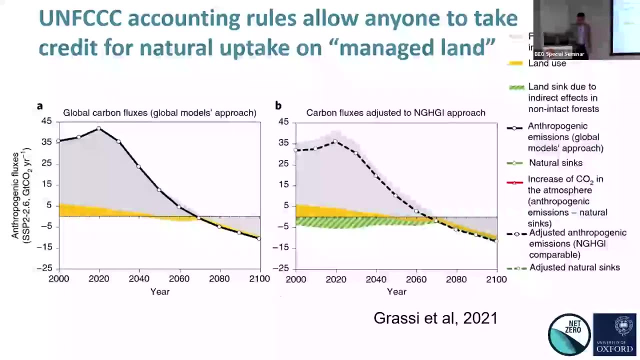 credit for this if it takes place on so-called managed land and suddenly lots of land is managed And we're seeing adverts like this one from a major fossil fuel company saying you could drive carbon neutral by planting in a forest. So just to give you a sense of the scale of this. 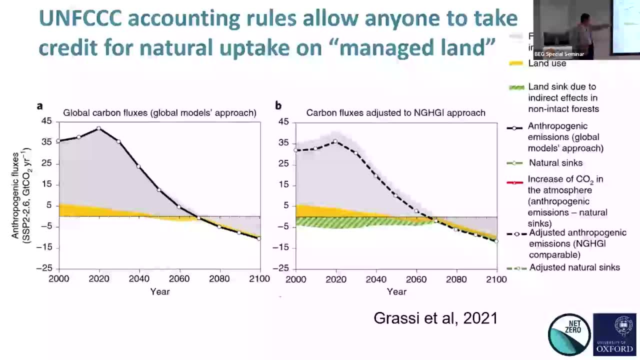 problem. This is the that green hashed curve. there is the sort of unaccounted for carbon And this is the ambiguous carbon at the moment. This is the carbon that, in one set of accounting rules, is regarded as a removal And in the way we, as the scientists, treated the problem, we regarded it as 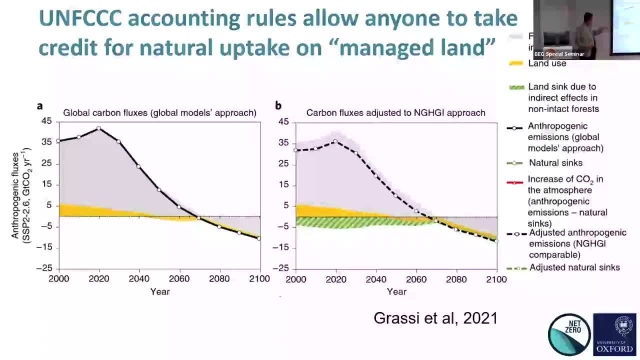 a natural response to the biosphere And if you look at this it doesn't look like that big a deal. It's like a small, small fraction of the problem And as we reduce emissions it seems to get smaller. But the 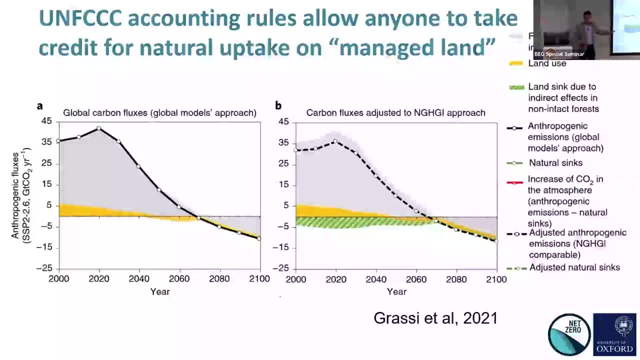 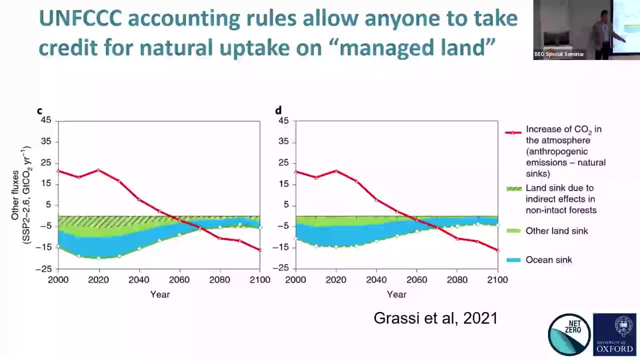 problem, of course, is that it's only part of what's being taken up by the land and oceans. So here it is, over, here again, with the other removals that are going on in the land and the oceans. And you know, Europe has just decided to include this in Europe's definition of climate. 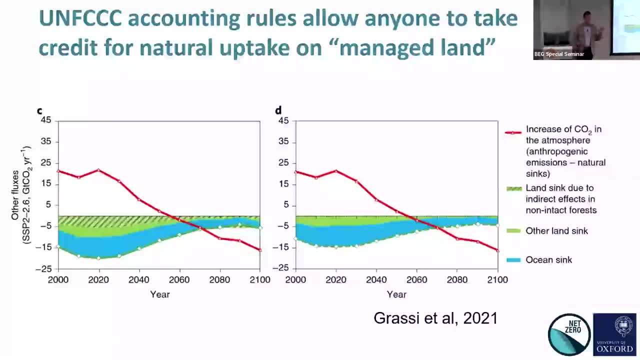 neutrality. So, despite having said for years that it would never do such a thing, other countries are waking up to this. No doubt Russia and Canada eventually will, And so well, maybe Canada won't, I'm sure. Well, whatever, I don't want to get too specific here, And you know there's already talk about managed 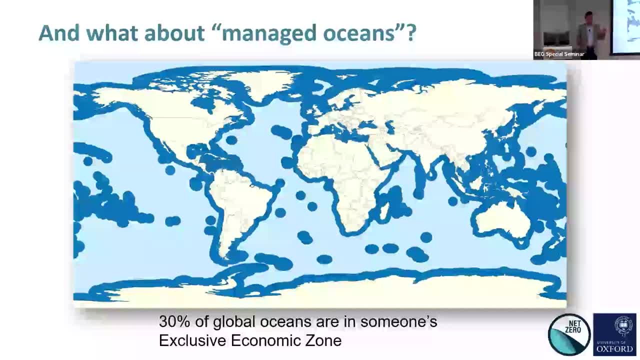 oceans. You know blue carbon is a big theme And if island states decide they want to take credit for the carbon being absorbed by the ocean around them, well, there's nothing in the rules to say they can't. But of course, if that happens, the net result is we'll achieve net zero. 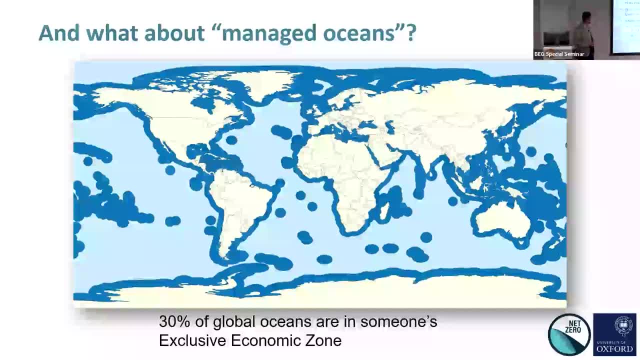 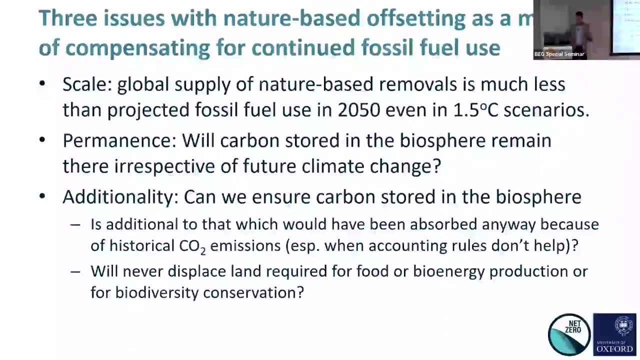 But we won't actually stop global warming, which was kind of the point. So these are the issues here. I mean, you know, everybody loves nature, based offsetting, but there's a scale problem, that the green line was a bit close to the zero line. There's a permanence problem And there's the 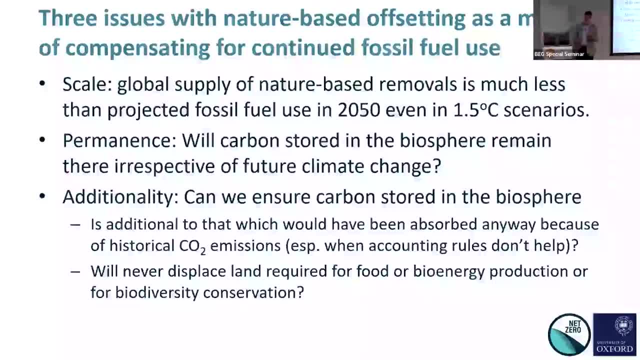 additionality problem that you. how can you be sure that carbon you're putting into the biosphere is actually additional to what would have gone there anyway, particularly when we're going to be short of land for food production? So if you're devoting land, 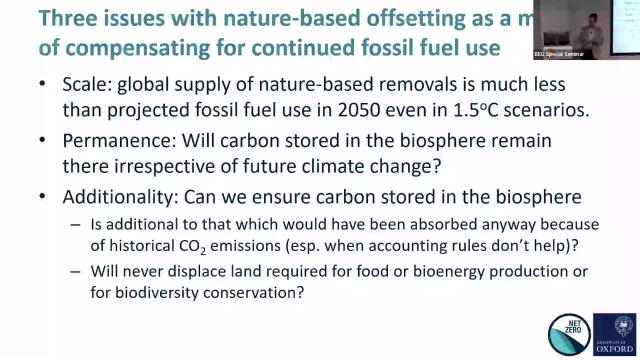 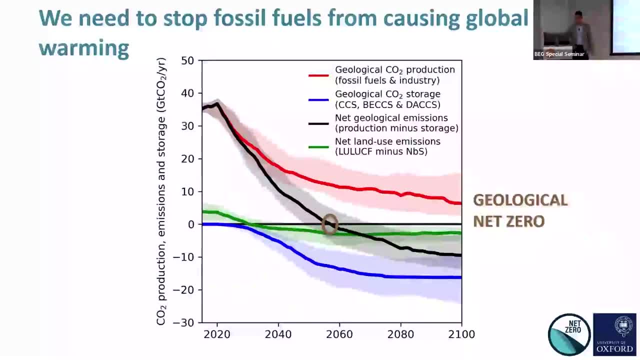 to absorbing carbon? how can you be sure that it's not simply displacing land for food production to somewhere else? So, to get back to basics, you know we need to stop fossil fuels from causing global warming, And that really means a balance between the red line and the blue line. This is what we. 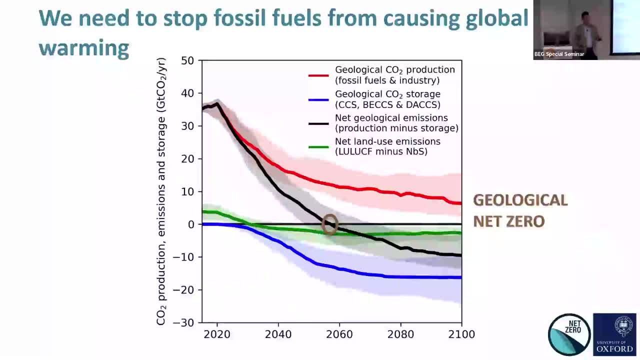 call geological net zero, where you're putting carbon dioxide back into the Earth's crust at the same rate that you're taking it out, that you're taking it out and generating it from continued fossil fuel use and production of cement. So the red line and blue line are equal And that's geological net zero. So basically, we need 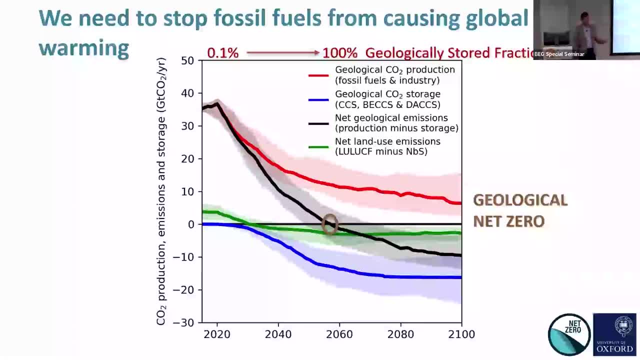 to get over the next 20 or 30 years. we need to get from where we are now, which is point 1% of carbon dioxide is put back underground. that's the 40 million tonnes per year. we need to get that up. 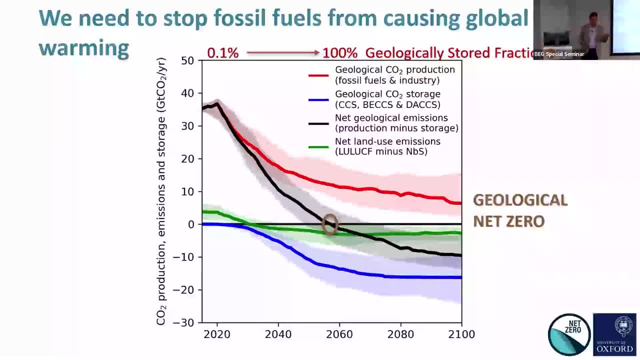 to 100%. So if we don't, that would mean 1000 fold increase in the rate of injection. If we don't reduce fossil fuel production at all, Actually, you can see, we do reduce it by around a factor of three or four. So it's only a 250 fold. 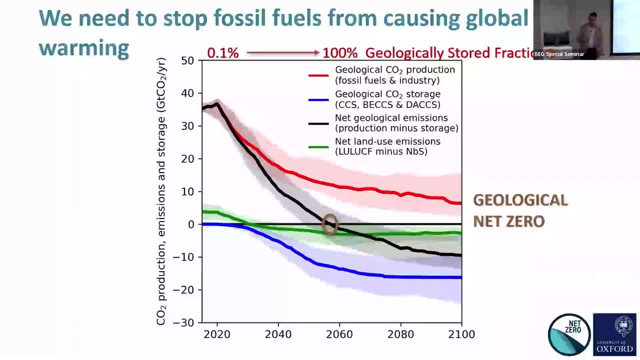 increase in the rate of which we store, but we need a maybe 1020 fold increase in the rate of renewable energy generation over this period. we need a 250 fold increase in the rate of carbon dioxide storage And I'm not going to. I'm going to move on from that. And if we look at what? 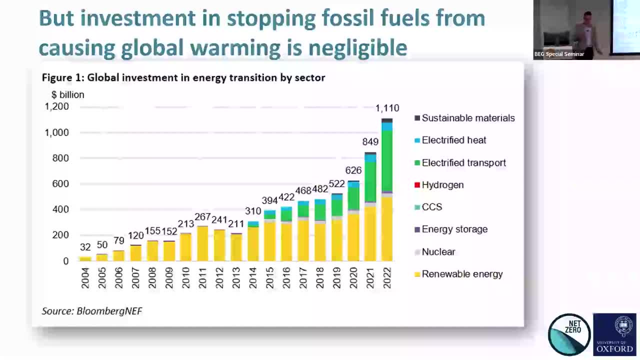 where the investment is going in different technologies for the transition. right now. this is from Bloomberg New Energy Finance. you can see there's only two of these. These technologies are directly relevant to stopping fossil fuels themselves from causing global warming. That's hydrogen and CCS. So hydrogen is relevant. if you're using hydrogen technology to, 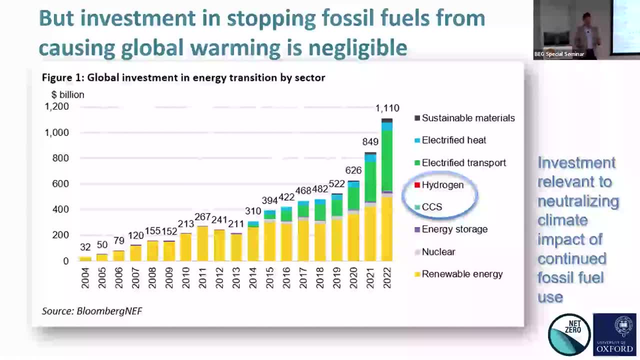 decarbonize fossil fuels And use hydrogen as an energy vector. if it's blue hydrogen, that's all relevant to avoiding, to preventing fossil fuels and causing global warming. Of course, carbon capture and storage is central to, and can you see on the well? you can't actually see on the graph where the hydrogen 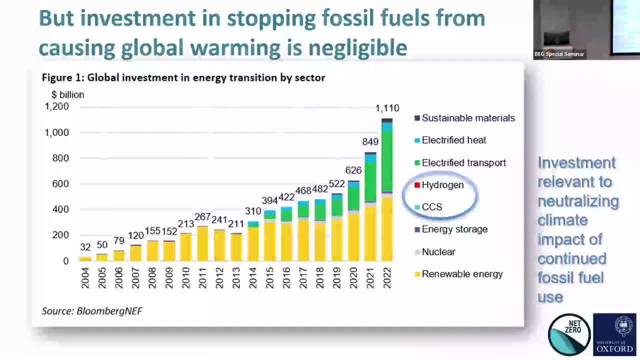 and CCS bars are that they're here? Okay, You can't even see them. And it's 25% of the solution and much more than 25% Of the cost, because this is the expensive 25% And it's getting none of the investment. 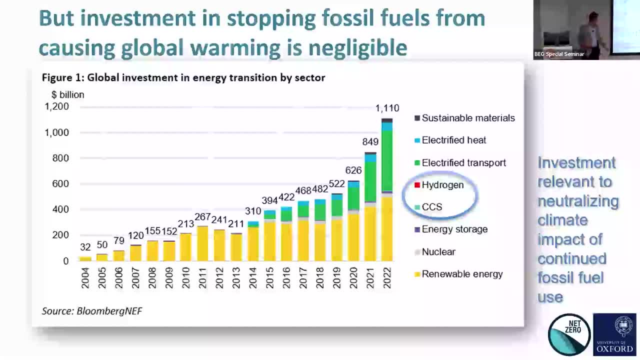 And nobody's talking about this. Indeed, Bloomberg, New Energy Finance almost celebrated it by saying, yeah, CCS has been technology. It's not getting the investment. That's a great thing. It's the biggest problem we've got at the moment And the reason is really straightforward Again. 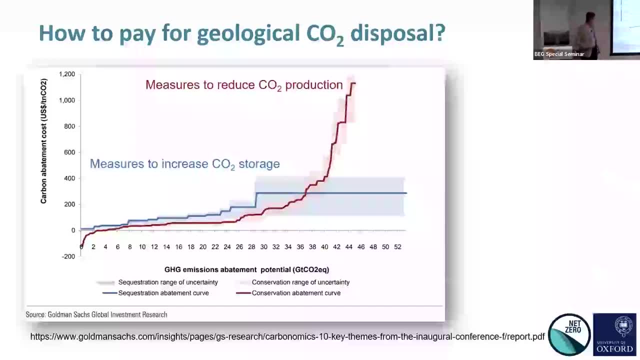 this is from a Goldman Sachs report, But I mean the basic point is, it's fairly obvious If you look at measures to reduce, this is one of these classic marginal abatement cost curves. the cost of reducing emissions okay, the more you reduce emissions. 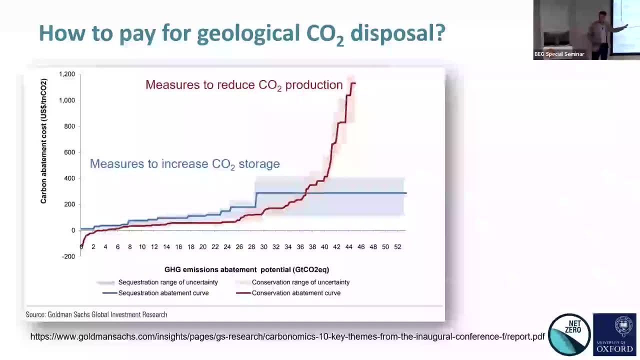 the more expensive it gets to reduce the next ton of emissions. And this shows you on the same graph: measures to increase CO2 storage in blue and measures to reduce the amount of CO2 we produce in red. And you can see that over a lot of you know halfway. at least it's cheaper to. 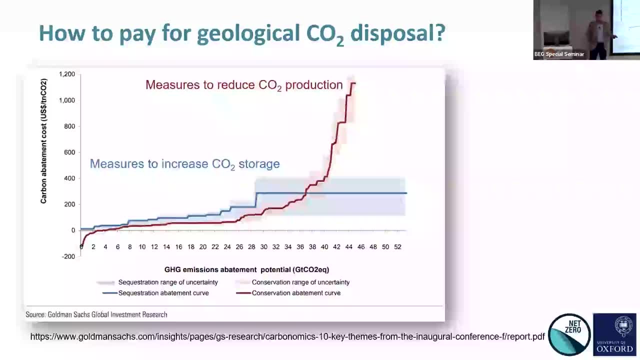 avoid producing the CO2 than it is to store it. Yes, carbon capture is expensive. It's much cheaper. There's so much of our fossil fuel. use is very inefficient. It's much cheaper to reduce our use than it is to store the CO2.. But then you hit a wall. Then you get to applications like cement. 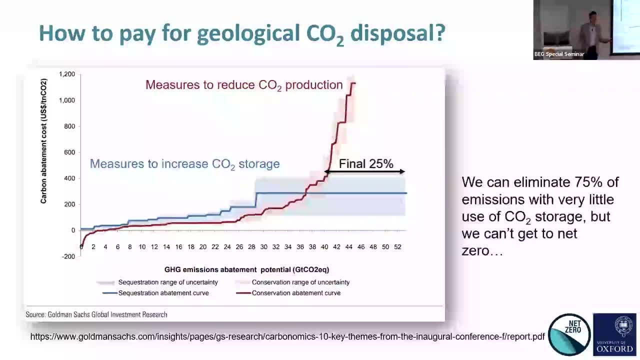 production, like aviation, where there is no alternative to using fossil fuels and there won't be an alternative in time. So we end up with the cost of reducing emissions becomes the cost of actually banning activities, And that becomes very, very expensive indeed. So it's that final 25% where we're absolutely counting on driving. 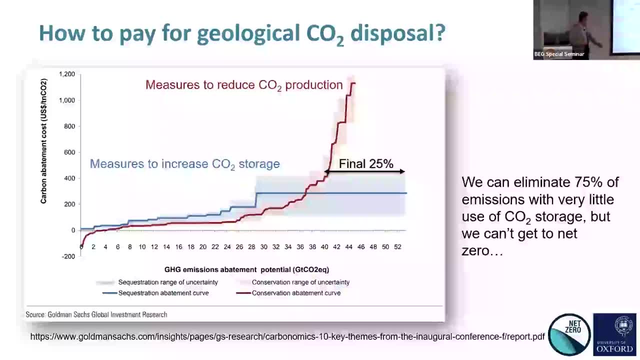 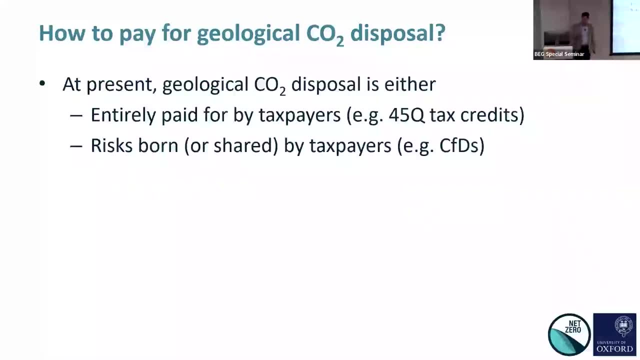 up our capacity for CO2 storage. So how do we pay for this? So right now, carbon dioxide disposal is either entirely paid for by taxpayers- which is the system here in the US, pretty much with these companies- Or at least the risk is borne by the taxpayers. So that's what in the UK we're doing. 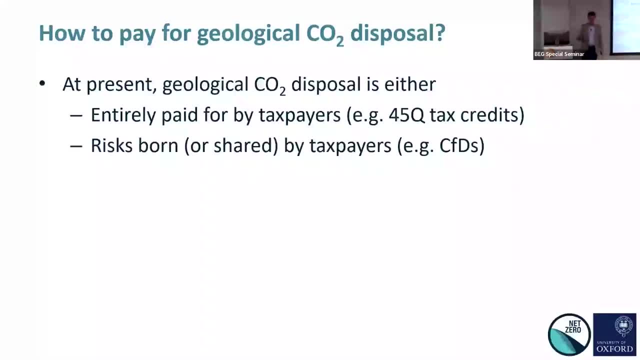 it entirely with public subsidy. In the European Union they're trying to build systems where there's at least a risk sharing between the private and public sector, But the public sector is completely on the hook on this. Neither of these mechanisms is particularly efficient at driving. 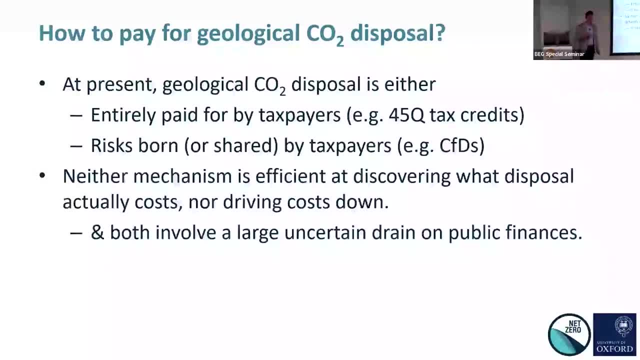 down the cost And that's, I'm sure, a lot of the reasons why we've not seen the cost reductions we would have liked to have seen in CCM- Yes, over the past 20, 30 years, And they both involve a big and very uncertain drain on public. 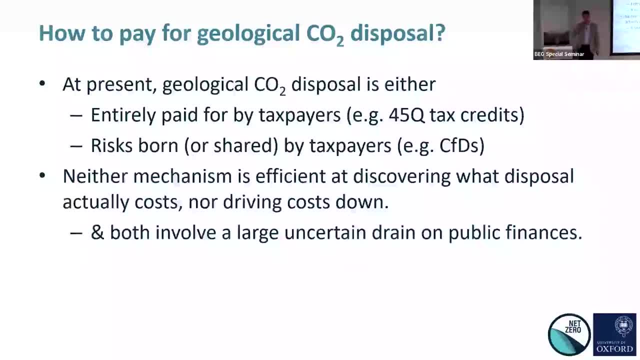 finances And I'm very concerned in the UK that climate policy is starting to become political And if we are dependent on public subsidy to drive the whole carbon capture and storage industry, another government will get in and just say: no, I'm sorry, we want to spend that money on. 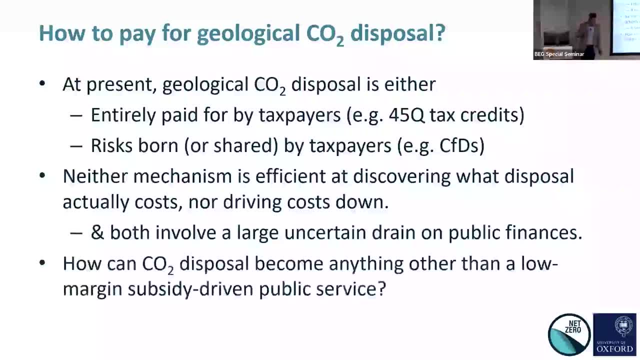 something else. So how can we? And also again, Texas, nobody likes public subsidies in Texas, do they, I mean? and so how can we change the narrative around this so that carbon dioxide disposal can become something other than a sort of low margin, boring, subsidy driven public service? And here's a suggestion for you to sort. 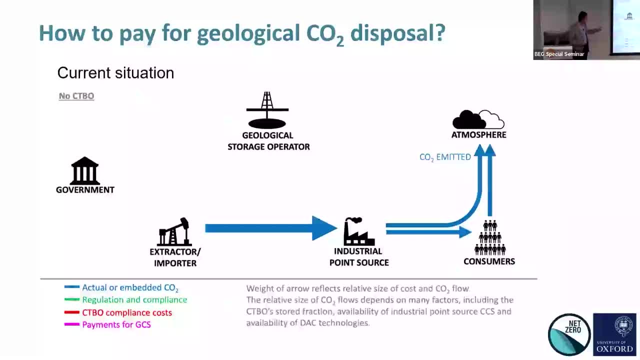 of take away as to how it could be done. So this is our current situation. Blue shows you the flow of actual or embedded carbon dioxide through the economy. It comes in from an extractor or an importer, It's sold to an industrial refiner or a factory that produces. 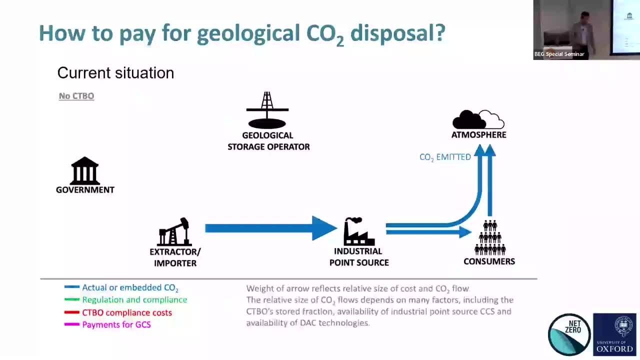 goods which are sold to consumers and it all ends up in the atmosphere Right now in Europe. so the point sources have an emission trading system imposed on them, So they've got. The only people affected by climate policy really are the point sources, So they're unhappy. The 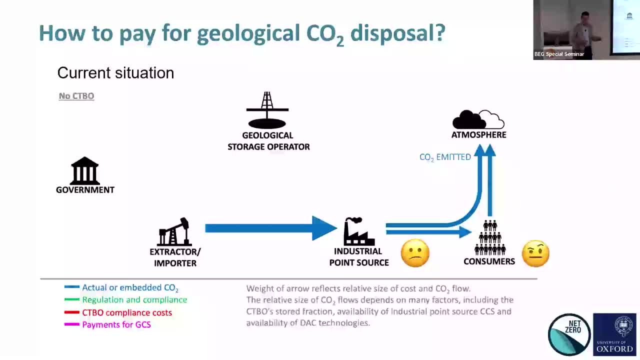 consumers are confused because they can't quite see what the point of this climate policy is. The atmosphere is sweating Over here. we have a geological storage operator who is sad and lonely because they have no business. I mean, there's no arrows pointing towards them, There's no business case for doing. 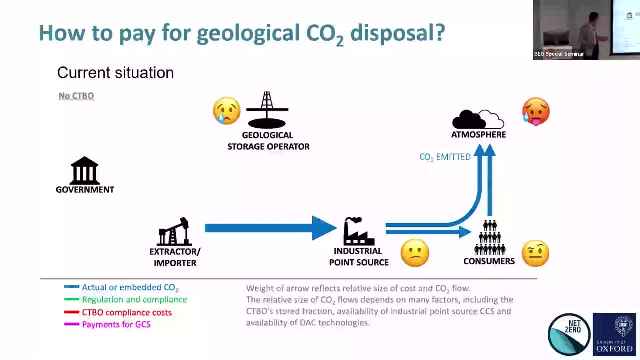 what they're doing. They've dug a hole, but there's no CO2 to put into it. The government's fast asleep and the extractor importer is laughing all the way to the bank. So we introduced something called the carbon. take back obligation. This is a policy mechanism that 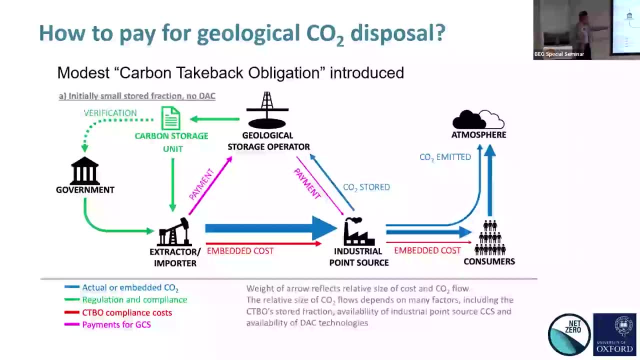 requires the extractor importer to produce evidence that some carbon dioxide has been stored, some fraction of the carbon dioxide that will be generated by the fossil fuels that they bring into the economy. A small fraction to start with, 1%, a few percent, And what then happens? Well, they obviously have to buy that from that carbon. 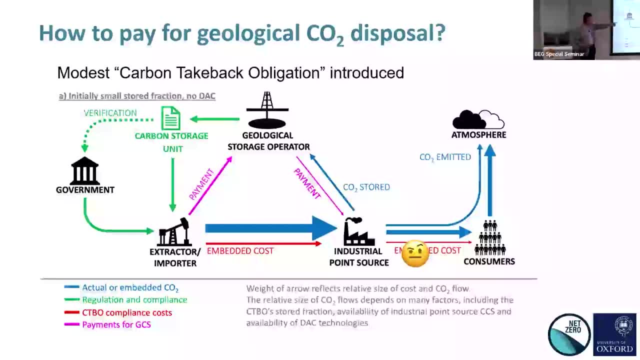 storage from the geological storage operator who has to get the carbon dioxide from someone else. They probably buy it from the industrial point source. but they're now intrigued because, instead of carbon dioxide being a liability, carbon dioxide becomes valuable. Carbon dioxide becomes a resource. 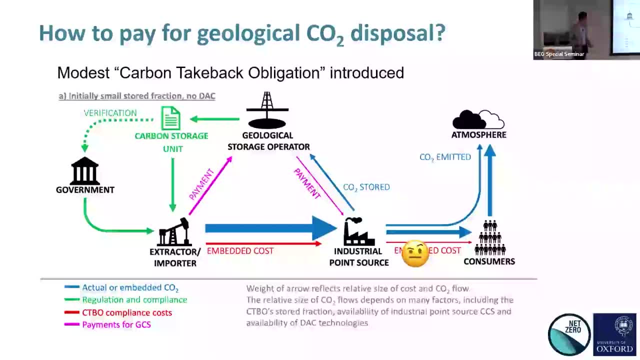 And it's worth capturing it because then you can sell it to generate these certificates. Consumers wouldn't notice because it's quite small still, this obligation. The atmosphere is still sweating. It hasn't made any difference to the flow of carbon dioxide into the atmosphere. 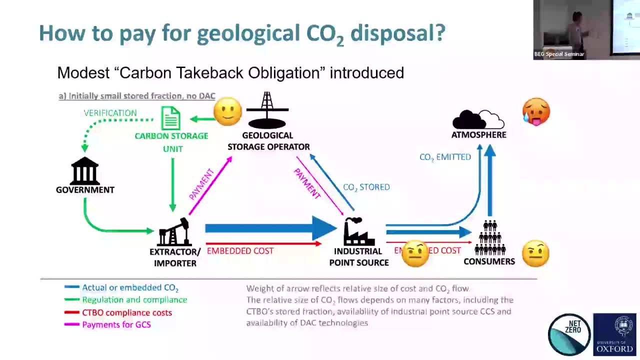 but the geological storage operator is now happy because they have a business. The government has its nerd glasses on because it's learning how to do this And, of course, the extractor importer is a cross because they now have a cost which they didn't have before. But hey, they have broad. 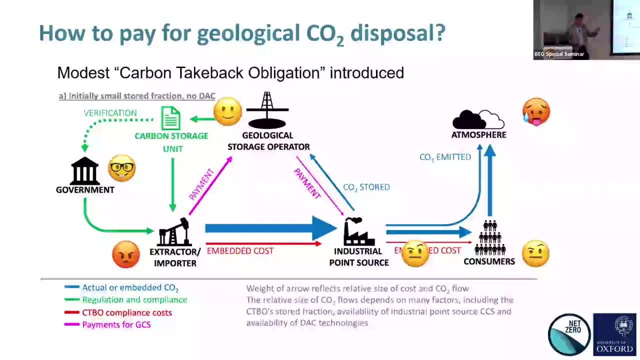 shoulders. OK, We scale up the stored fraction, We increase this fraction. The industrial point sources are now happy because they're being paid a lot for their CO2.. Consumers are probably still confused. The atmosphere is feeling a little bit better because we've now got a new element, that's. 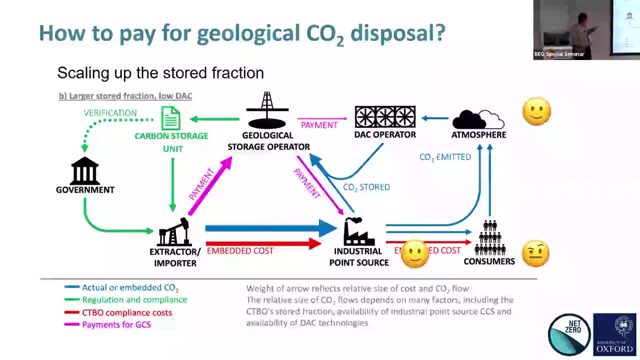 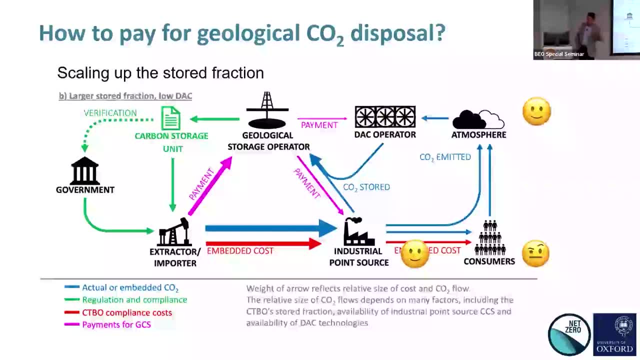 to recapture CO2 from the atmosphere in order to generate certificates fast enough to satisfy demand for these storage certificates. They're doing really well And the government is still getting good at the job And the extractor importer is maybe feeling a little bit better. 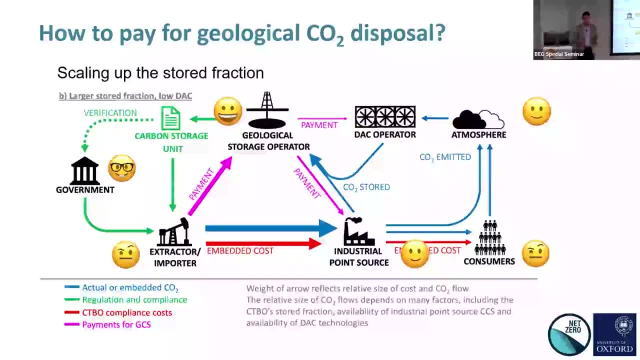 about things because they're starting to see how this actually could provide them with a sustainable future. Finally, we get to net zero. The industrial point source is happy because they're selling all their CO2 and not having to pay into the emission trading system- Consumers. 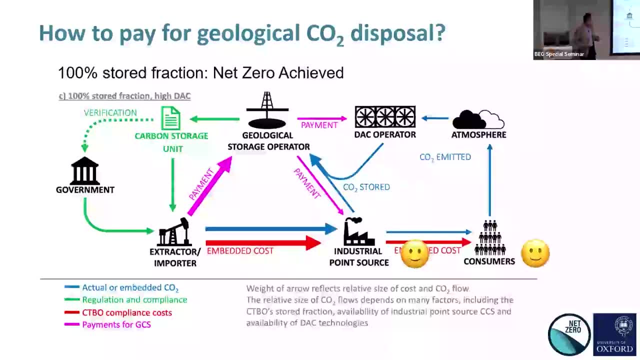 are happy because we stopped global warming. The atmosphere is breathing a sigh of relief, The geological storage operator is still making loads of money, The government is feeling awesome because it's stopped global warming And the extractor- importer has saved the planet. There are other ways of doing it. Here's the emission trading system that we're counting on. 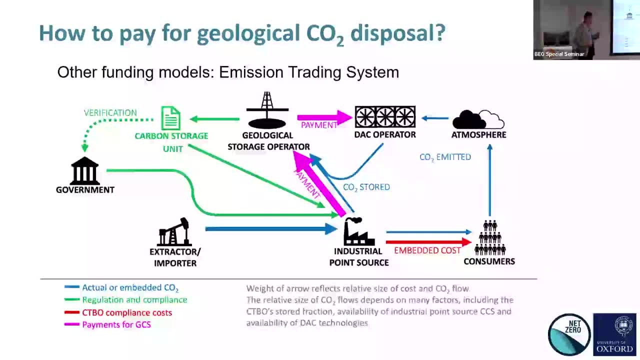 in Europe where the government just requires the industrial point source to get rid of CO2.. That makes the industrial point source very cross. The whole burden gets put onto them and they head off to China. And that's what we're doing, And that's what we're doing, And that's what we're doing, And 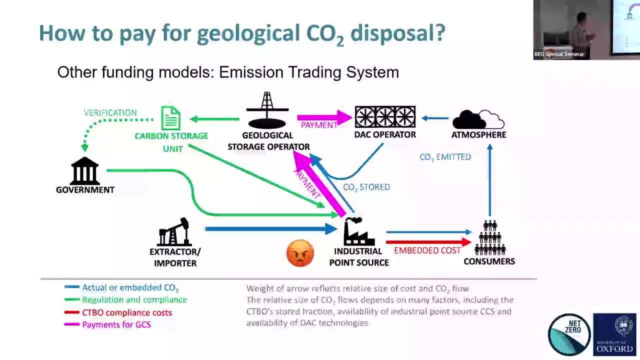 nobody wins. The other option, which is kind of your model over here, is a tidal wave of government cash is thrown at geological storage operators, which means the government's cross because it's spending a lot of money and consumers are cross because their taxes are being spent on very rich. 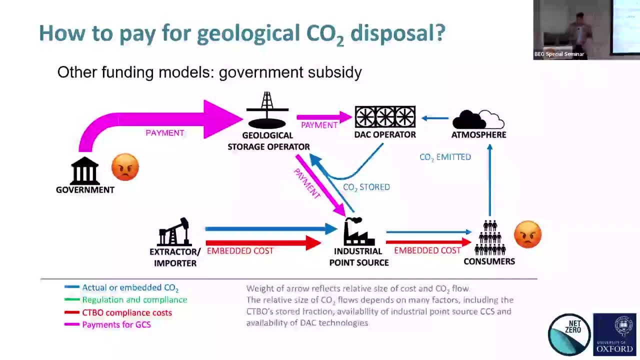 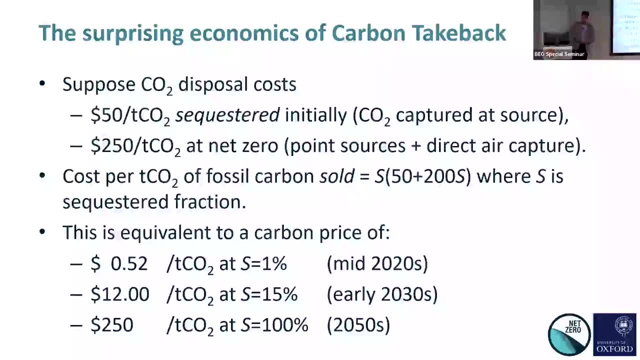 companies And again, I don't think it's a sustainable model. We need to think about this because the economics are remarkably interesting, If you think about what it costs to dispose not of all of the carbon dioxide associated with the use of fossil fuels. initially, we have to get there. 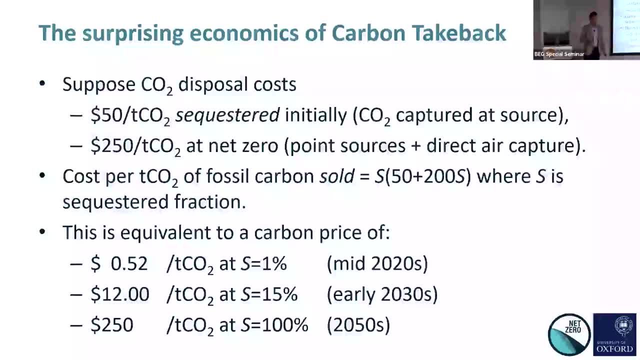 eventually, But initially you start small. start at 1%, 10% in the 2030s And 100% by 2050 is what we should be aiming for. The cost of that that would be reflected in the cost of fossil fuels to. 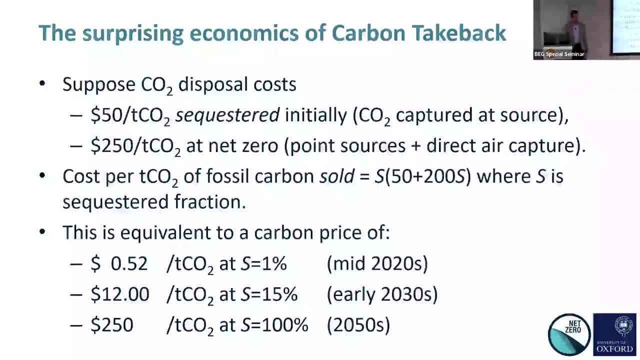 the consumer is perfectly manageable. It's not, you know, an immediate penalty that would put people off climate policy. It would work. it would get us to net zero. it's a simple single regulation that would get us all the way, And you know, if you just think about what it means, even in 2050, and this is 20 years away- 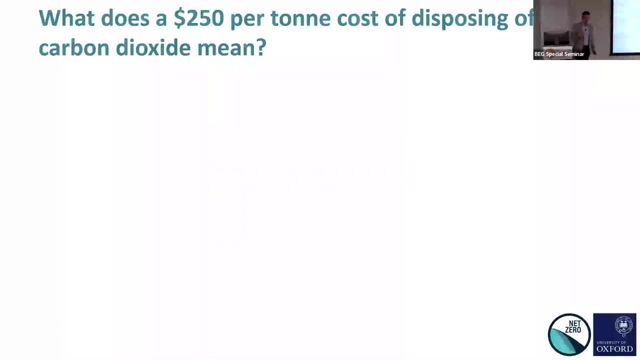 25 years away. we need to be in a situation where every tonne of carbon dioxide generated by any continued fossil fuel use is being captured and put back underground, And by that stage, probably a lot of it would be having to be recaptured from the atmosphere and put back underground because 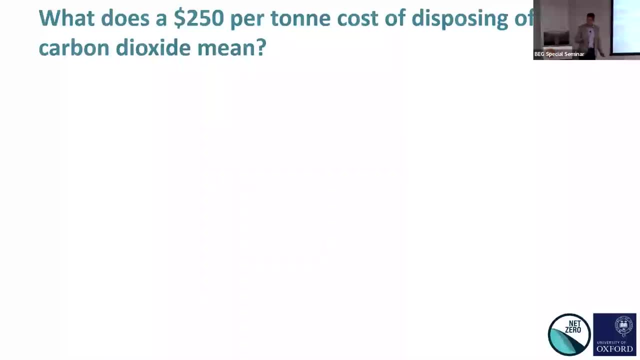 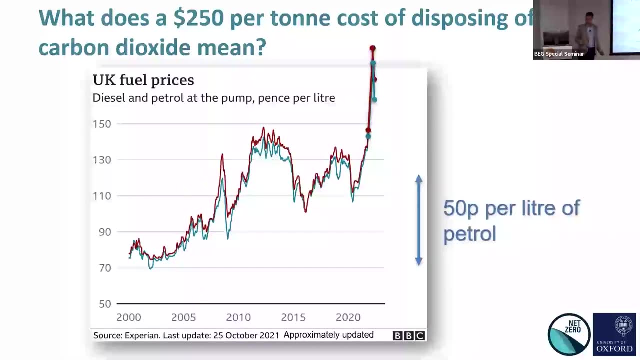 many of the applications we'd still be using fossil fuels for will be mobile. we won't be able to capture the fossil fuel at source. It's 50 pence per litre of petrol. Okay, apologies to the unit here, But that's how that compares to UK fuel prices over. 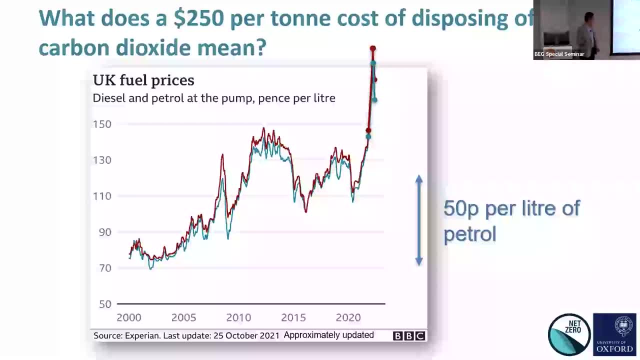 the past 20 years or so. So you know less than the gyrations in fuel prices we had during the Ukraine crisis, since the Ukraine crisis blew up, And also, more relevantly, less than the overall trend in fuel prices we've seen since 2004.. 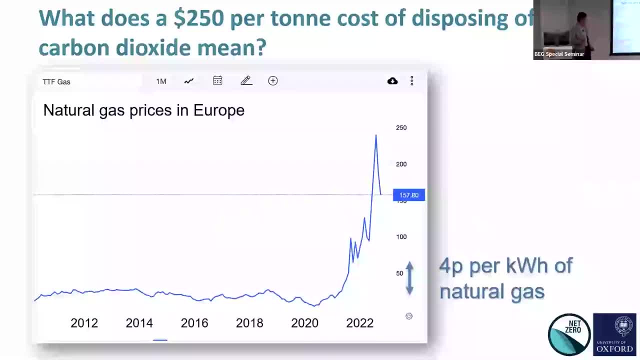 And that's over a similar period. It's even more strikingly small compared to the fluctuations in natural gas prices we've seen in Europe over the past couple of years, And the point is, while nobody's liked these high prices, the world hasn't come to an end, Whereas 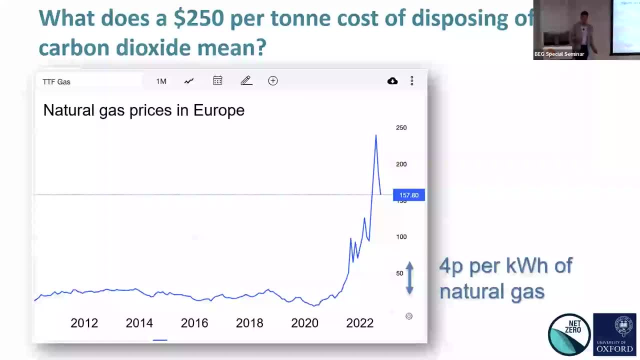 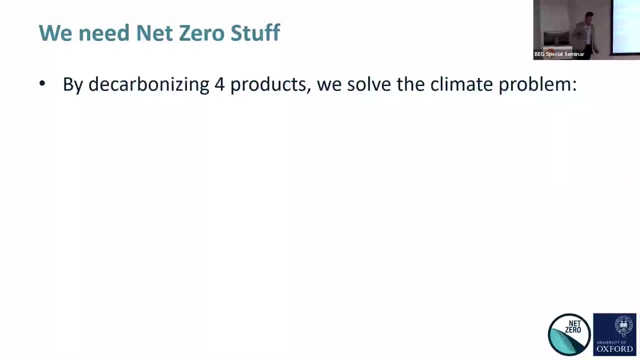 not to make it sound too much like an environmentalist here- if we carry on putting the CO2 in the atmosphere. well, one day, Anyway, we need just to sum up: we need net zero stuff. We think too much about this problem, as we need net zero systems. 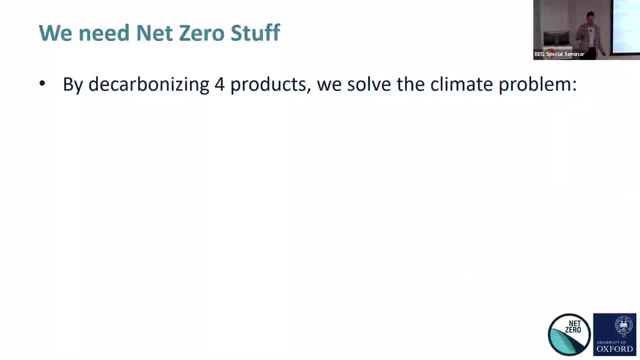 or we need net zero companies. No, we need net zero commodities And we really only need four commodities to be made net zero: Coal oil, natural gas and cement. If we stop those four commodities from causing global warming, we largely solve the problem. 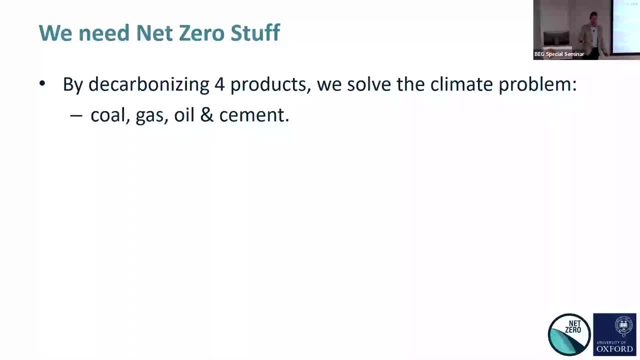 Yes, we need to stop deforestation. We need to do that anyway. Yes, we need to have a sustainable food supply system. Yes, but we need that anyway. okay, These are the big ones. We've got to stop these products from causing global warming And in each case. 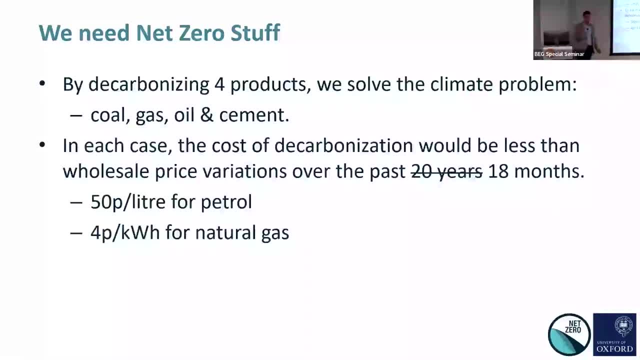 the cost of decarbonization would be less than wholesale price variations over the past 18 months. Just remember this: We didn't save the ozone layer by changing consumer attitudes to personal hygiene. We fixed the stuff in the can And we have to take the same approach. 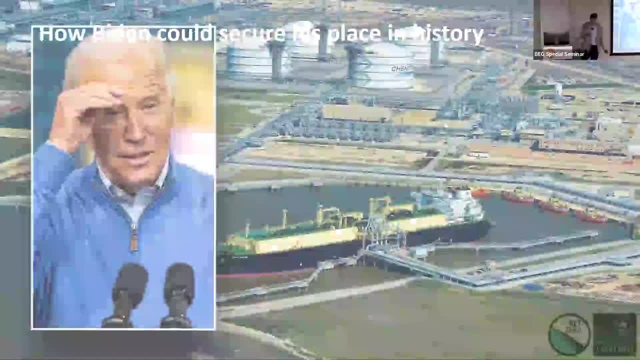 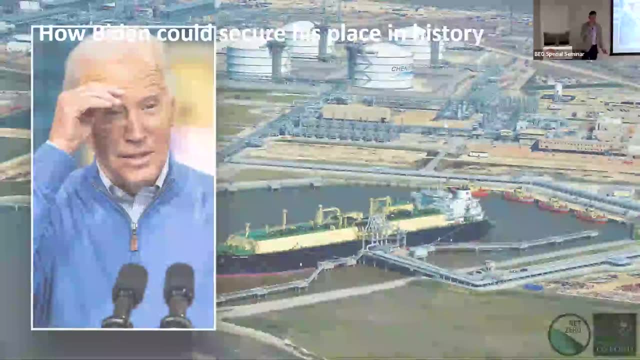 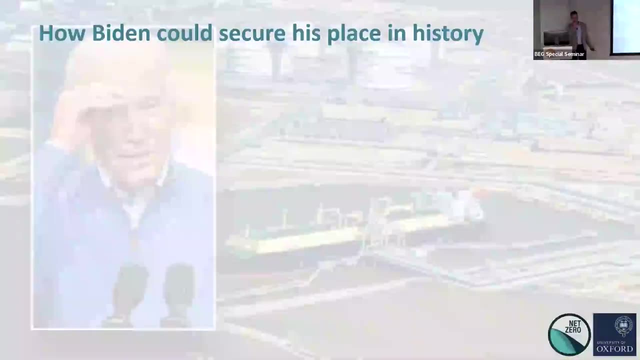 I think, to dealing with climate change. So this was this morning. I was thinking about how could this map on to the current situation the US is in, how Biden could really secure his place in history. Just imagine he sat in the Oval Office and said, look, the United States will be the. 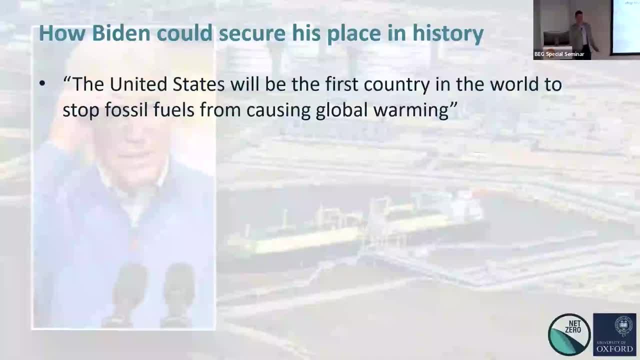 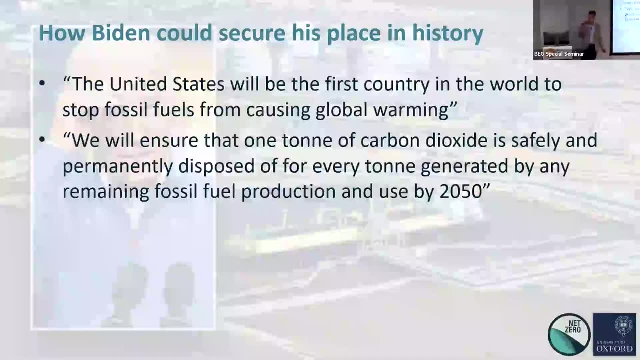 first country in the world to stop fossil fuels from causing global warming, And we're going to do by ensuring that one ton of carbon dioxide is safely and permanently disposed of for every ton generated by any remaining fossil fuel production and use by 2050.. New licenses for any new 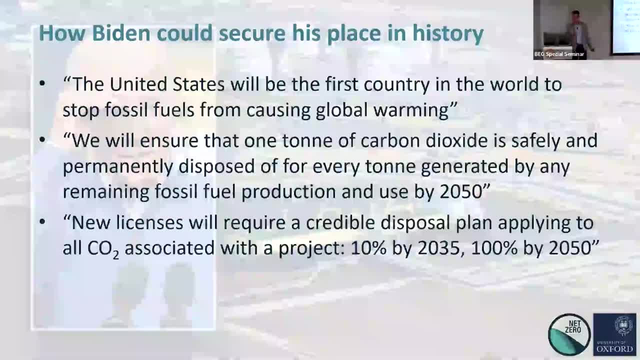 infrastructure and extraction will require a credible disposal plan applying to all the CO2 associated with the project: 10% by 2035,, 100% by 2050. And we're going to require all our trading partners to do the same. So come on, Europe, China, Australia, you've all got to step up. 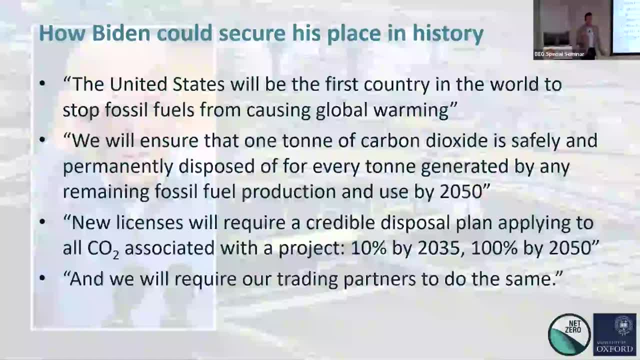 That would take less than 30 seconds and it would completely transform the world, Because there's no way the European Union would be able to not go along with that approach. Everybody would kick up, everybody would complain, But at the end of the day, the logic is absolutely. 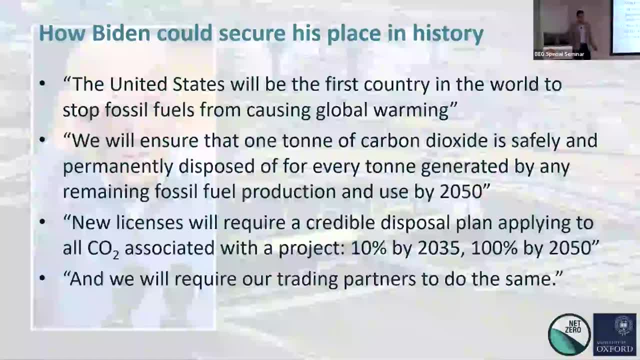 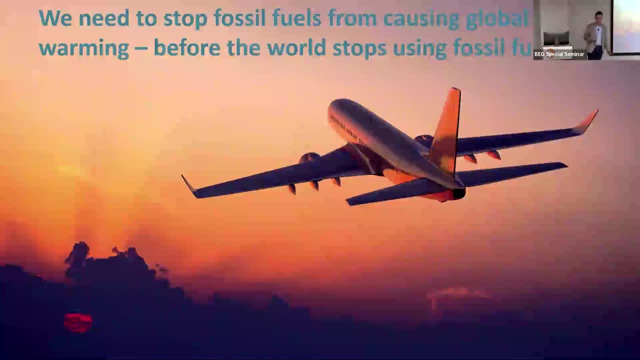 unassailable. Interestingly, most of the environmental justice movement would immediately attack it, which is really depressing, But it would solve the problem, Because we need to stop fossil fuels from causing global warming before the world stops using fossil fuels. And just to sum up with a punchline, quoting a 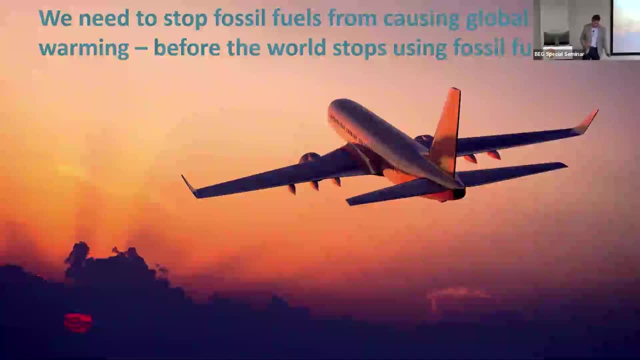 I quoted Sultan al-Jabbar earlier. I'll quote an earlier journalist. Sheikh Jamani from the Saudi oil minister in the 1970s, Commented that the Stone Age didn't end because we ran out of stones. the oil age won't end because we run out of oil. 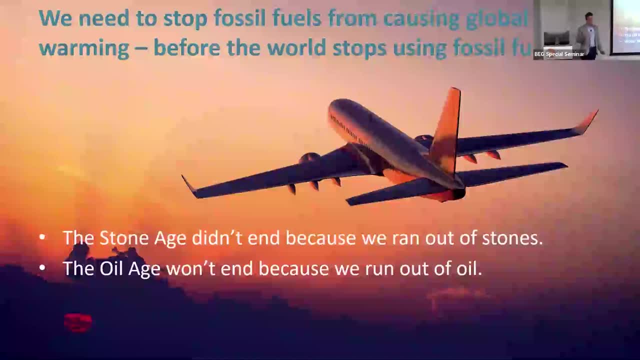 And we have to recognize and accept that global warming must end before we stop using fossil fuel. I'm sure you've got some questions. Thank you for that awesome presentation, as always. I love it. Okay so questions. Okay so questions. 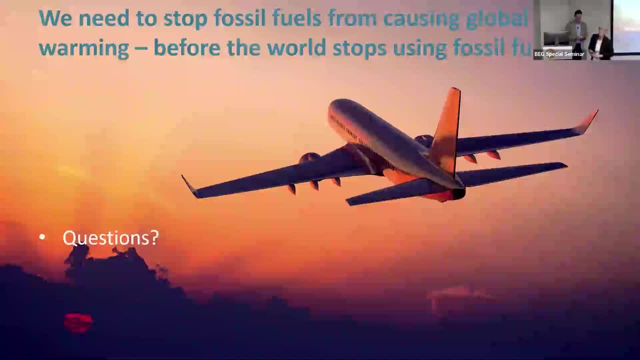 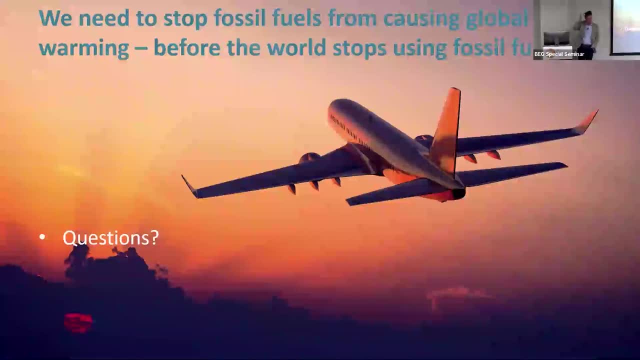 And indeed actually a couple of students of mine have actually now set up a little NGO, Carbon Balance. They're actually sort of campaigning for this for essentially producer responsibility. They're actually sort of campaigning for this for essentially producer responsibility for the fossil fuel industry, and this is what it is. extended producer responsibility is what we're talking about. They're actually sort of campaigning for this- for, essentially, producer responsibility for the fossil fuel industry, and this is what it is. extended producer responsibility is what we're talking about. They're actually sort of campaigning for this for, essentially, producer responsibility for the fossil fuel industry, and this is what it is. extended producer responsibility is what we're talking about. They're actually sort of campaigning for this- for, essentially, producer responsibility for the fossil fuel industry, and this is what it is. extended producer responsibility is what we're talking about. They're actually sort of campaigning for this for, essentially, producer responsibility for the fossil fuel industry, and this is what it is. extended producer responsibility is what we're talking about. 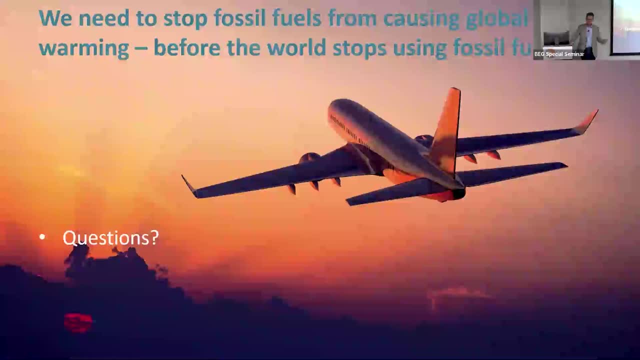